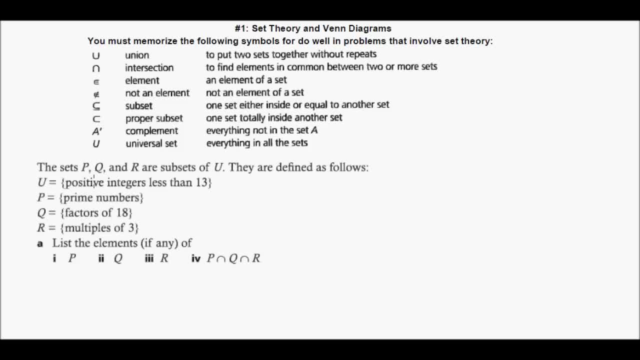 right there. it means not Universal set, that means everything in all the sets. Okay, so the best way to do this is just to let's start and do it So it says the sets P, Q and R are subsets of U defined as follows: Okay, so positive integers less than 13 is. 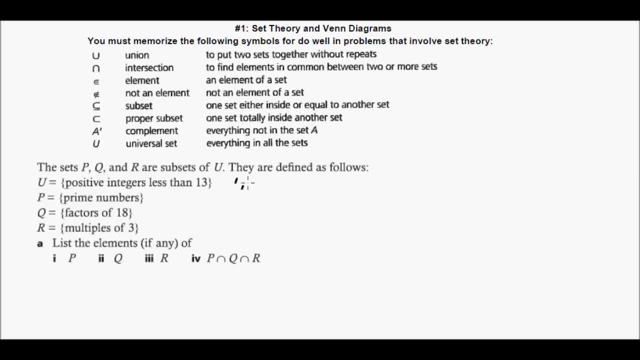 U. Okay, I always like to write that out, So that's just going to be, you know, 1,, 2,, 3,, 4,, 5,, 6,, 7,, 8,, 9,, 10,, 11, 12.. Okay, Now, you know, make my bad set brackets, like I. 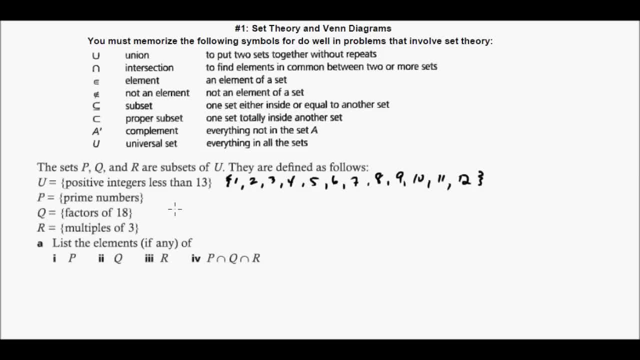 always do Woo, Okay. Now the prime numbers. Remember, one's not a prime number. One's not a prime number, Okay. so they want us to list the elements of P, Q and R, So I'm just going to do them. 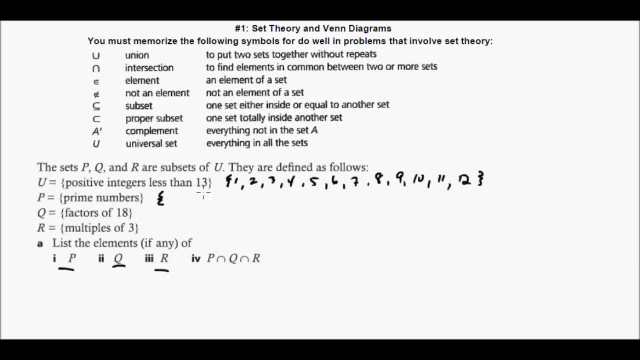 right here. Okay, so no one's not a prime number. So we start with 2,, 3,, 5,, 7, and 11.. Remember, the prime number just has two factors: one in itself, Factors of 18.. Now, with that, 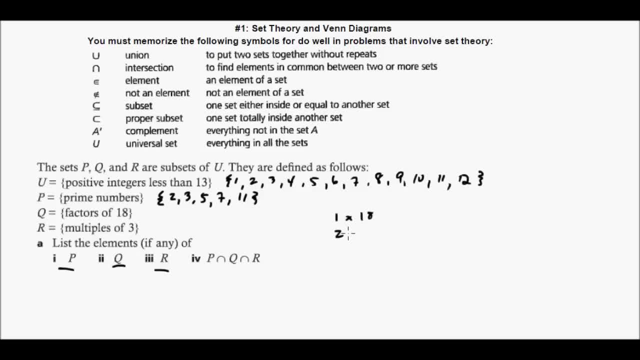 I would just go like this: 1 times 18,, 2 times 9,, 3 times 6.. So which ones are below 12.? Well, it's going to be 1,, 2,, 3,, 6, and 9.. So we will go 1,, 2,, 3,, 6, and 9.. Okay, 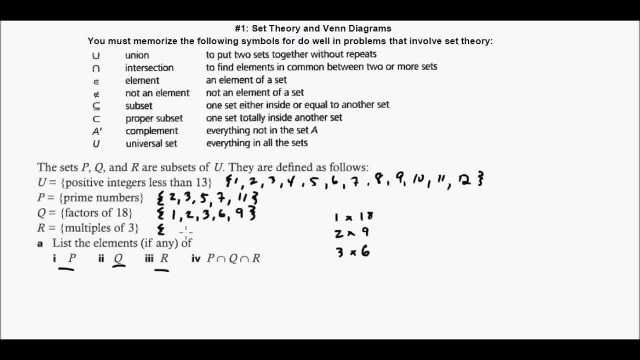 And then multiples of 3.. Multiples of 3 is just skip counting. So we'll go 3,, 6,, 9,, 12.. And we're good to go Now. this here says they want the intersection of P, Q and R. Okay, 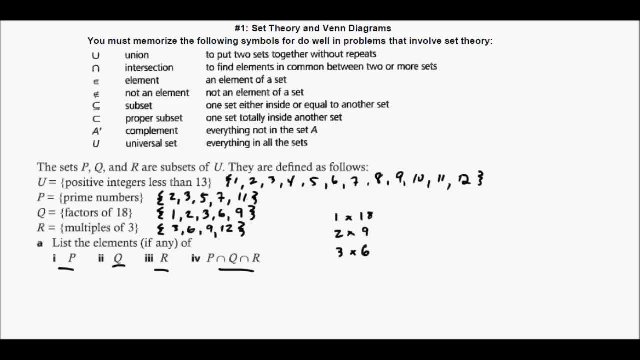 Okay, So the intersection of P, Q and R. Well, let's look what they have in common. Just looking here: Well, they all have a 3.. Okay So, 3,, 3, and 3.. Anything else? 5,, 7,, 6,, 9.. 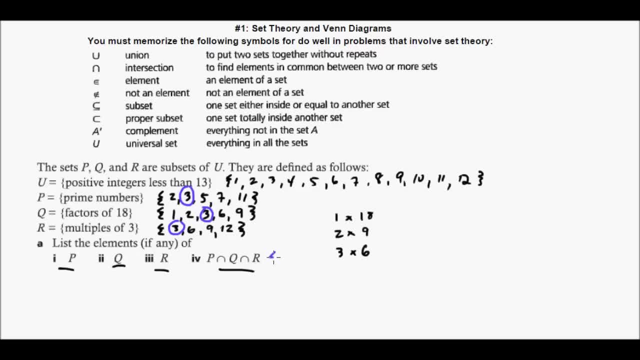 6, 9.. No, these don't have a 6 or 9.. So it's only 3.. So that's your answer, right there. Okay, So it's 3.. All right, So let's move on from here. Okay, For part B, it says draw: 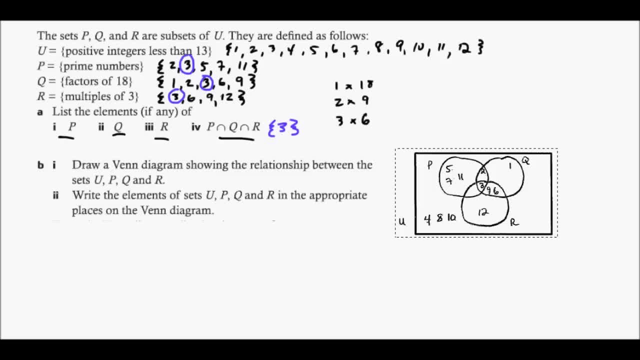 a Venn diagram showing the relationship between the sets U, P and Q, U, P, Q and R And write the elements. Okay, Well, I've already done this right here, So let's just take a look at this real quick. What 3 is you always in a Venn diagram? you always work out You. 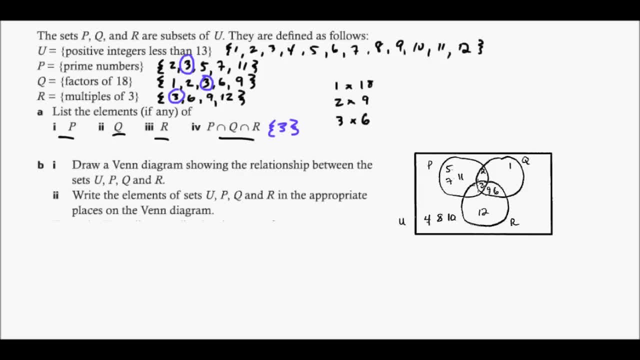 know, I think of LFMAO, You work out, You work out from the middle. So 3, I would put that in first. Now P and Q have a 2 in common And then P, you know, has 5,, 7, and 11.. And 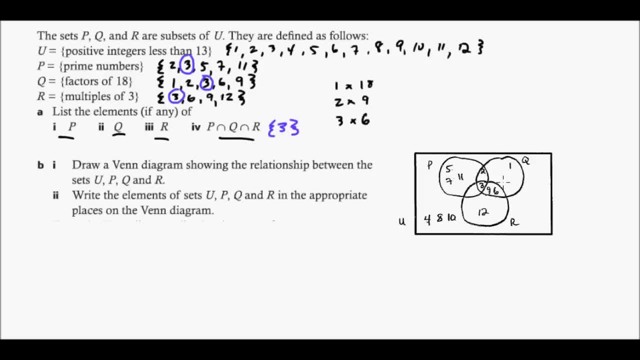 that's only in P, And then Q has 1.. And then Q and R have 3,, 6, and 9 together. And then don't forget to put all the ones that are not in either set. You need to put those out. 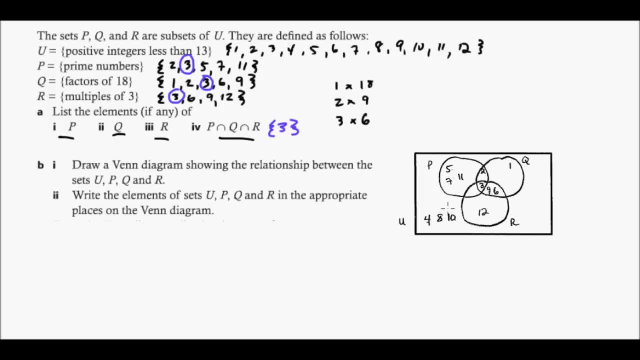 there. So 4,, 8, and 10 are out there. You know, just go through one thing at a time. I would just go 1,, you know 2,, 3,, 4, and then just put them in, And it's pretty straightforward. 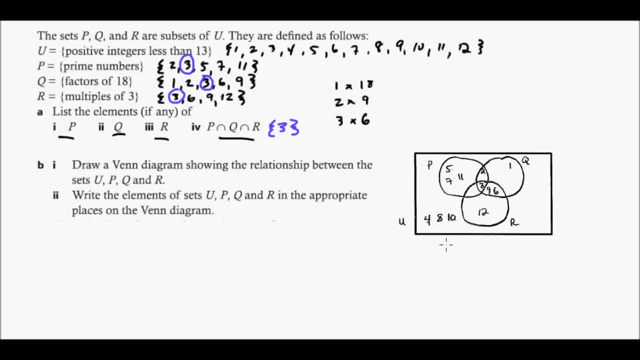 Most kids get this right. So what they're going to ask us to do now is they're going to ask us to shade some things here. Okay, Well, first they're actually going to say: from the Venn diagram, list the elements. 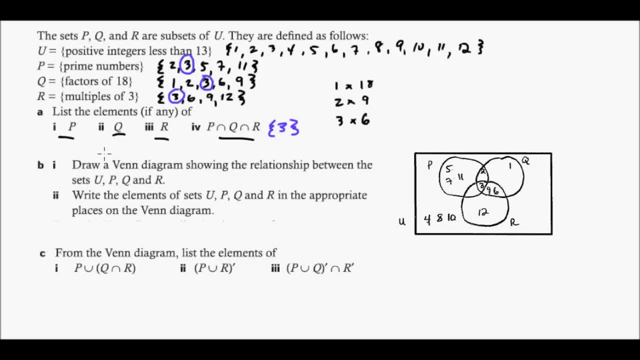 of P, union intersection Q and R. So P is going to be this whole circle right here, this whole P right there. Now the intersection of Q and R is right here. Okay, So if we, you know, if we look at this, this is a union problem. Okay, So we have, you know, P and 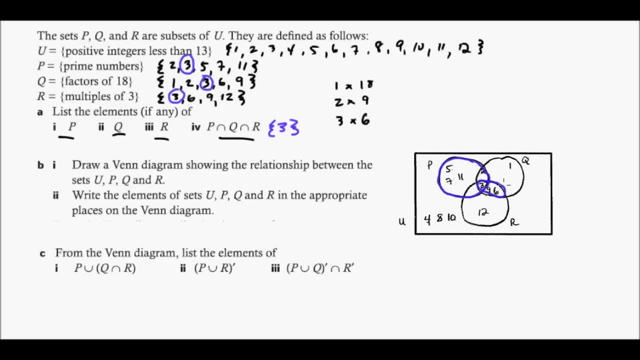 then we have R right here. Now it's a union, So we're just going to list all those right there. So we got you know. I mean I'm going to put them in order, but you don't have to 5,, 6, it makes it easier on the person grading. 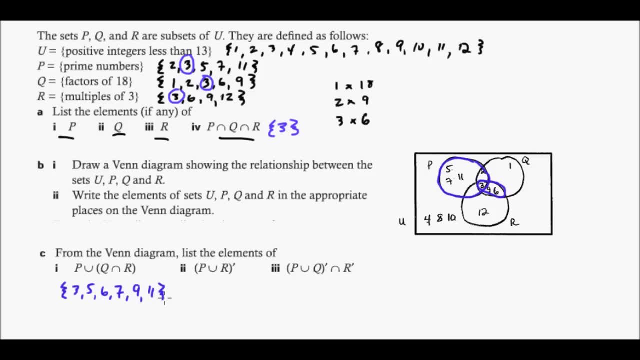 7,, 9, and 11.. And just make sure I have all those 6.. 1,, 2,, 3,, 4,, 5,, 6.. Oh shoot, there's a 2 there. 2 also, I almost missed one, So a 2.. Okay, So we're good to go on that one. 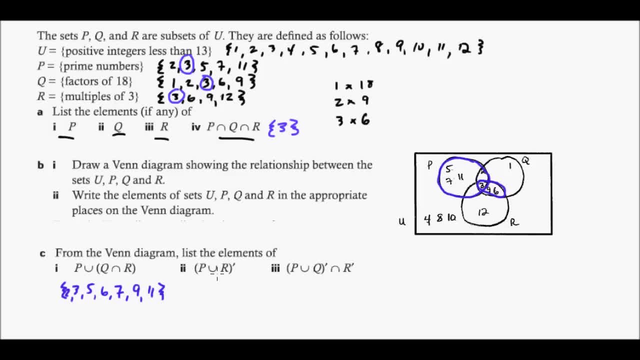 Okay, Now, not P Union R. Okay, So P union R is right here, So they're saying everything that's not P union R, So you know what they're looking for. is you know? not P union R, So they're. 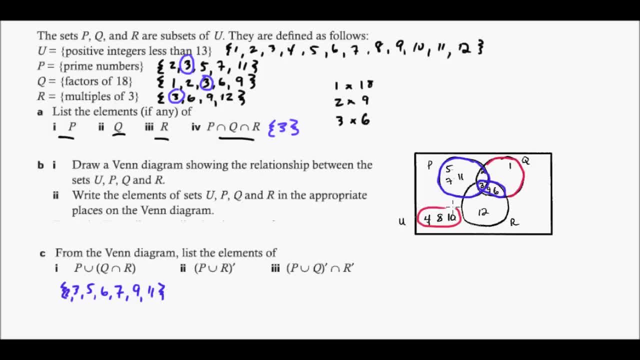 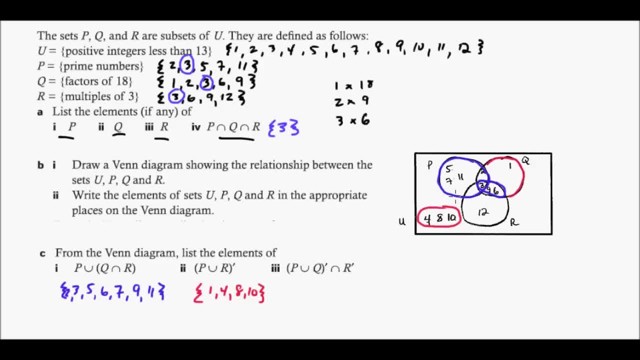 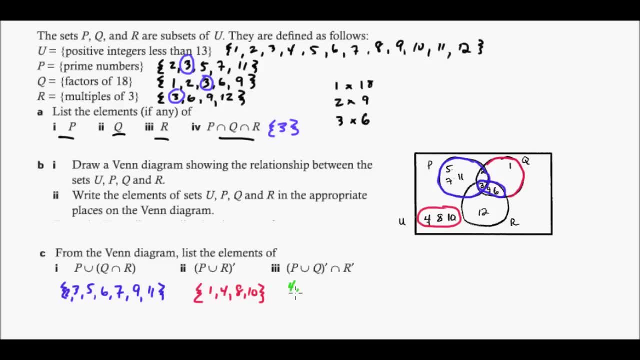 q would be, you know, 4, 8, 10 and 12, and then that's the intersection with not r. well, not r is, you know that's a lot of them. it's um, you know 4, 8, 10, the outside ones, plus all p and q, but we, we know it's. 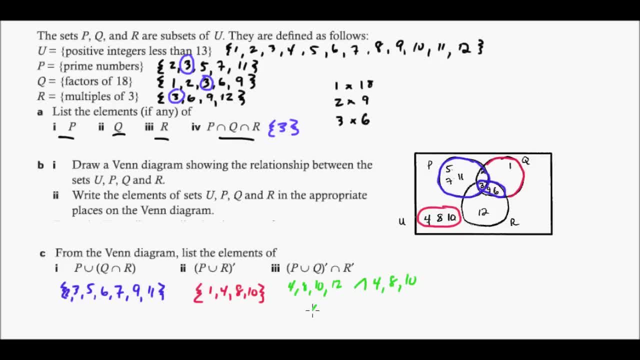 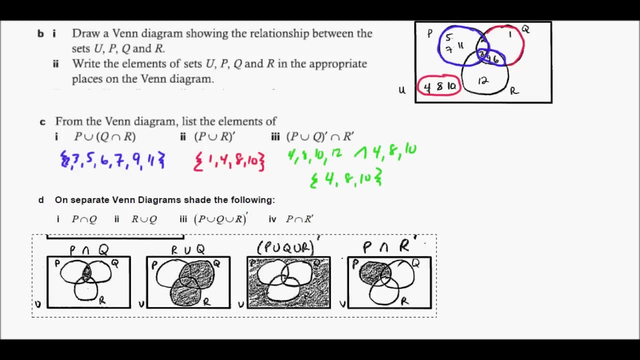 not going to be part of that. so, if we just look at this, it's going to be, you know, 4, 8 and 10. that's going to be our answer. okay now. uh, now we'll do a little shading. okay, so, on separate venn diagram, shade the following: now i, i did these on a piece of paper and i just pasted them in here. 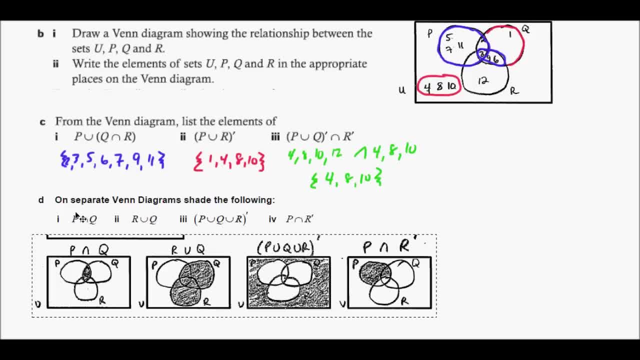 for the sake of time. so the intersection of P and Q. Okay, so PQ, just remember you have to shade both of them. so it's you know right in here That one's not too bad. Union of Q and R. well, that's just going to be all of Q, you know. 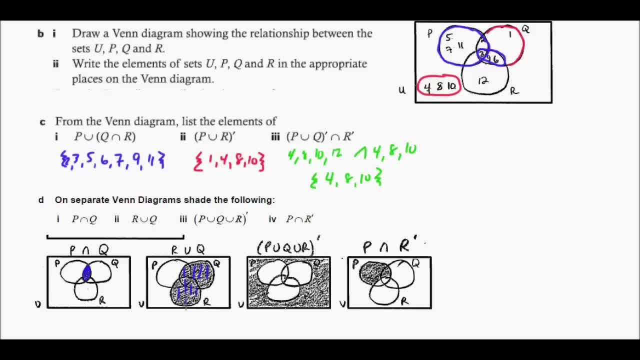 right here and all of R. Okay, so we're good to go there. Those are pretty easy. Now, union of P, Q, R. that would be all three circles, but it says not, so that's just going to be the outside. 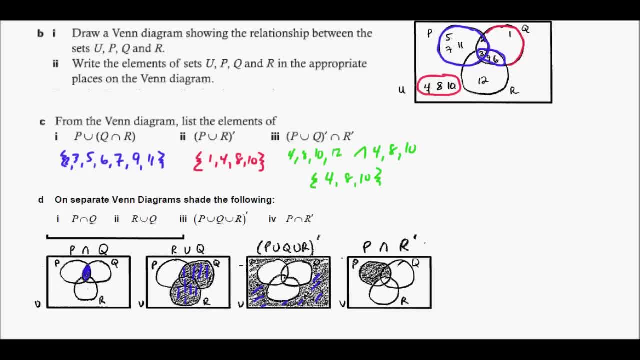 right there, Okay, and you know. finally, the last one: P intersection, not R. So not R is going to be all the stuff out here and it's intersectioned with P, so they have to be in the same thing. so it's just going to be that right there, Okay. so you know. shading in Venn. 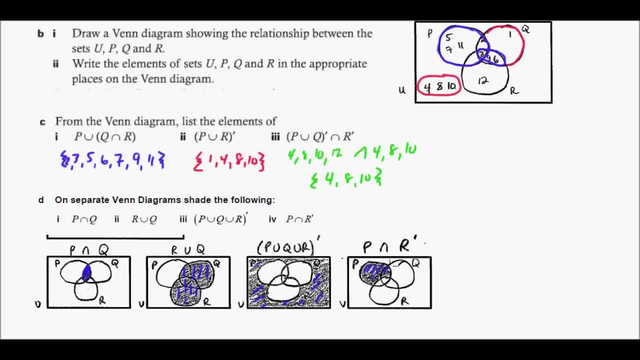 diagrams. it's not that bad, You know, if you can do it properly. these are some easy points. This might be worth, you know, I don't know- four points and another fourth say like eight points, eight marks. 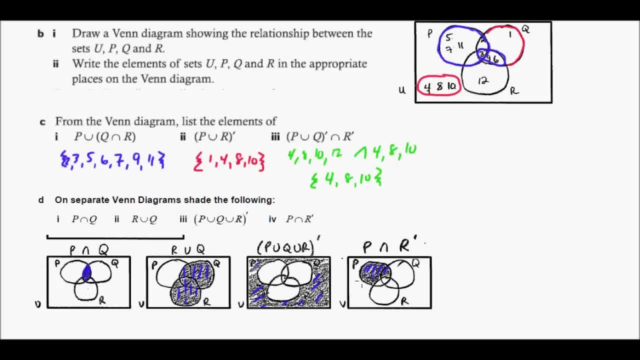 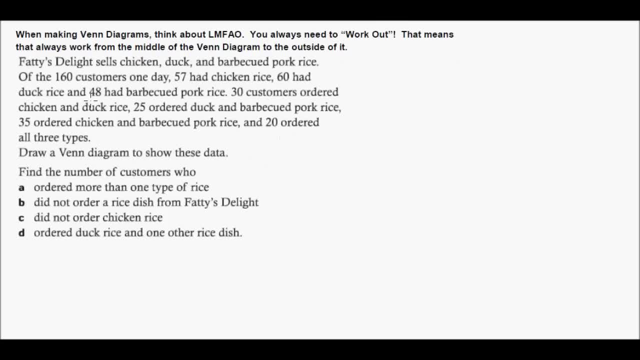 on a test, which is kind of a lot, Okay. so what I'm going to do on the next couple problems is make a couple more Venn diagrams, just to make sure we're square on that, Okay, so you know. 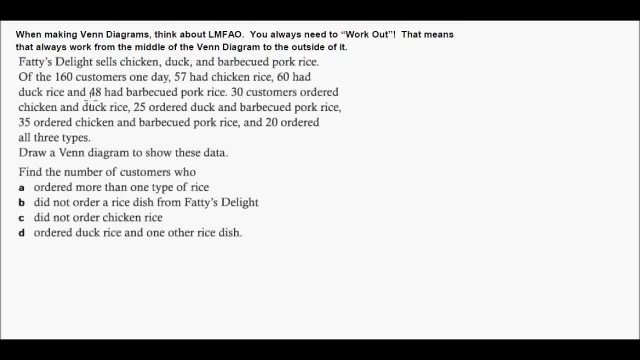 I said this before, but it bears repeating. When making Venn diagrams- think about LMFAO- You always need to work out, which means you always go from work from the middle of the Venn diagram to the outside of it. So we're going to make a Venn diagram for this data here. 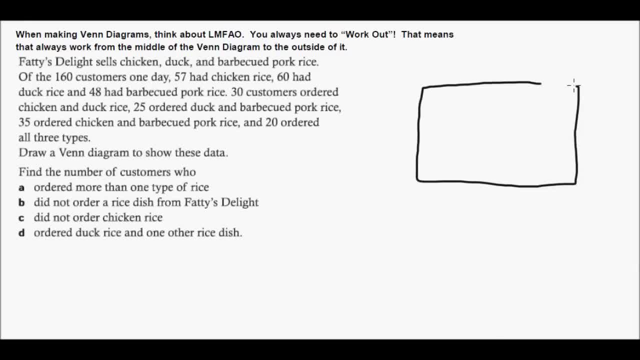 Okay, and I'll make it nice and big and not very neat. You know, always make sure you know you draw your rectangle around. that That's actually, believe it or not, in every mark scheme. that's worth one point, And I have kids who just won't. 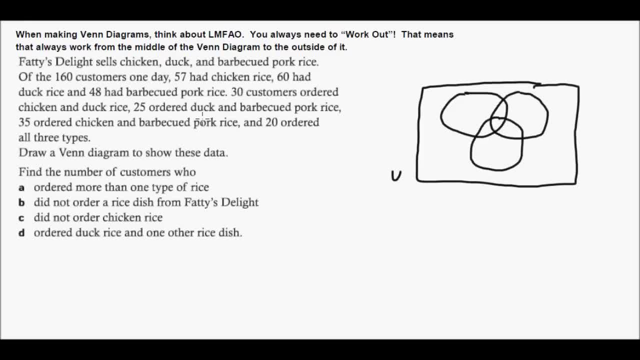 do that and they get dinged every time. Okay, so it says Fatty's Delight sells chicken. Okay, they sell chicken duck and you know, barbecue Pork rice of 160.. 57 had chicken rice, 60 had. 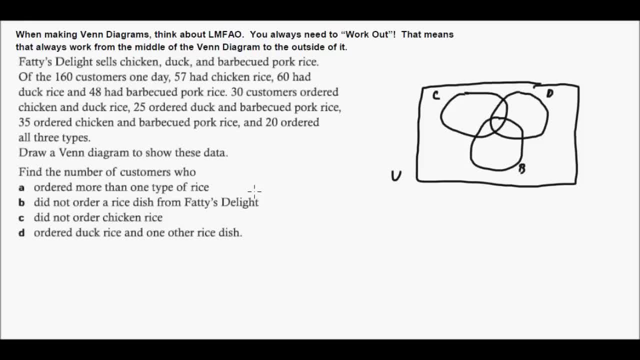 duck rice: 48 had barbecue pork rice: 30,. ordered chicken and duck: 25 ordered duck and barbecue. blah, blah, blah, 35 ordered chicken and okay, whatever, All right. so this is the important part, is you know? starting from. 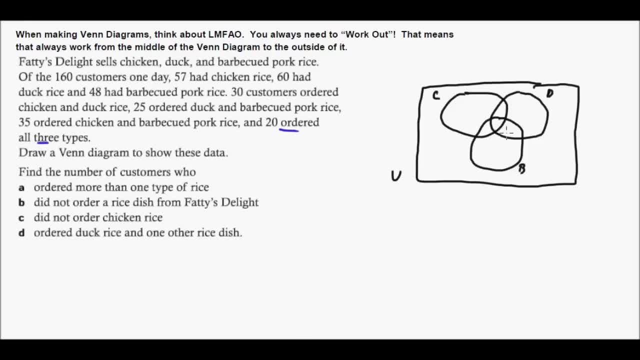 like I said, the middle. So 20 ordered all three. Okay, so we're going to put 20 right there, Okay. now the thing is it says you know, 35 ordered chicken and barbecue. Okay, well. 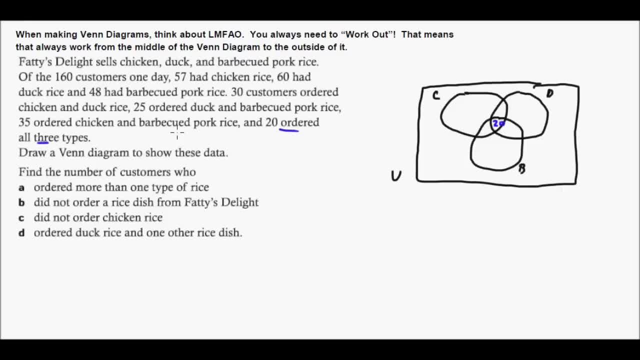 okay, we don't put a 35 there, you know, because if they said chicken and barbecue only, then we would put a 35, but we don't, So we need to actually do 35 minus 20, which is 15.. So we need to put that there. Okay now 25 ordered duck and barbecue. 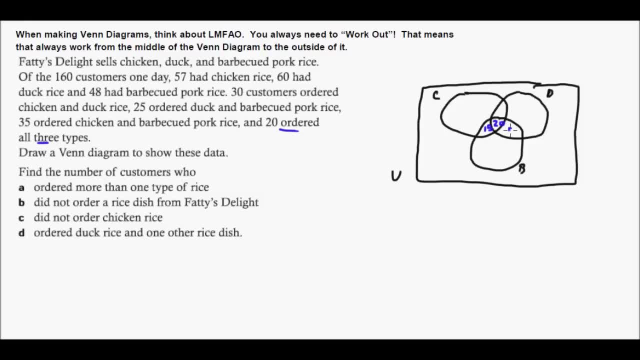 Duck and barbecue. so it's 25 minus 20, which is 5.. Okay, and then 30 ordered chicken and duck, so that's going to be 10.. 30 minus 20 is 10.. Okay. now 30 ordered chicken and duck, So 30. 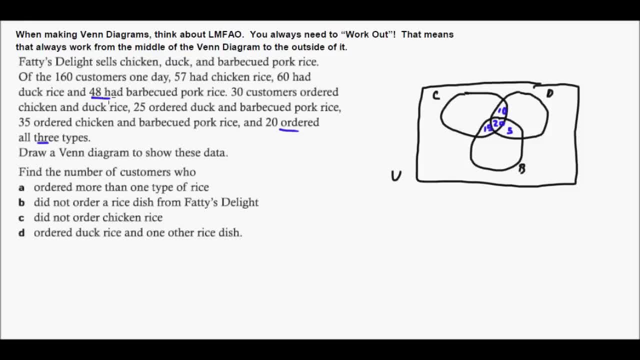 ordered chicken and wait, hold on, whoops, sorry. 40, 48. ordered barbecue pork rice. Okay, well, this is, you know, 25,, 40, you know. so this one's going to be 8 right here, And if you add all these up it's going to equal. 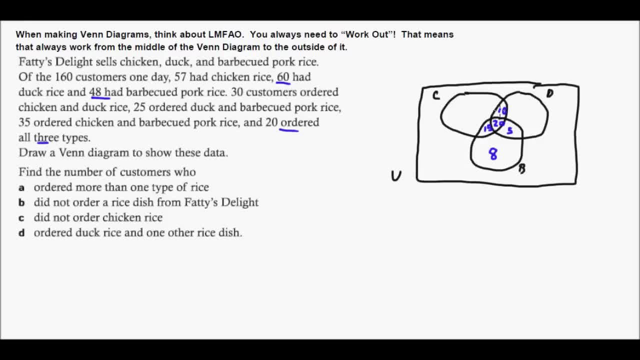 48.. 60 had duck and barbecue. so that's what? 30,, 35,, so that's going to be 25, to get to 60.. And then what do we have? 57. So we have 30,, 45,, 57,, so that's going to be 12.. 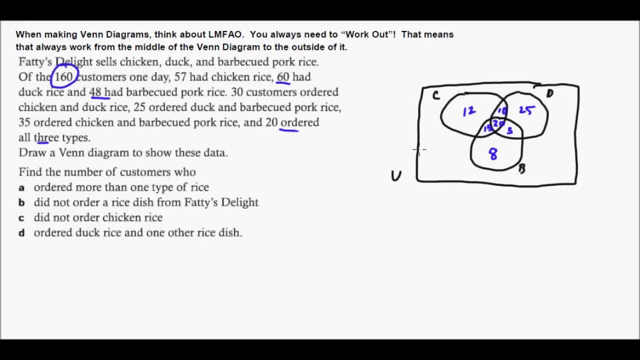 Now, if you add all those up, we need, there's 160 customers. We want to know how many didn't have rice. And if you add all those up, we need, there's 160 customers. We want to know how many. 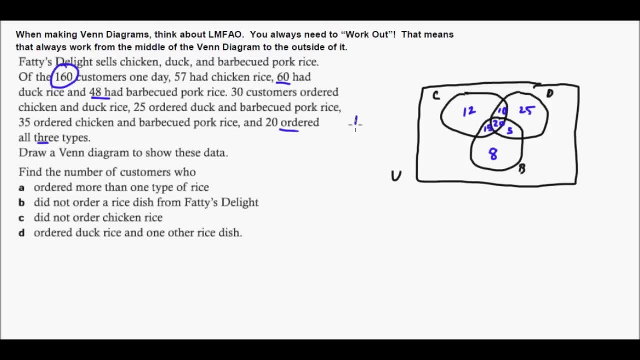 didn't have rice, And if you add all these up it adds up to 95.. So if you, you know, if you do 160 minus 95, you get 65. And that's, you know the numbers. that didn't have anything, So you know. 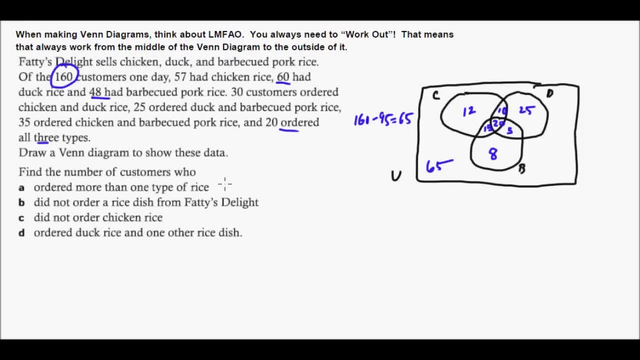 you want to make sure you're good with that, So find the number of customers. so let's answer these questions. Who ordered more than one type of rice? Well, more than one type of rice is just going to be. you know anyone who ordered two, or anyone who ordered three. So it's you know. 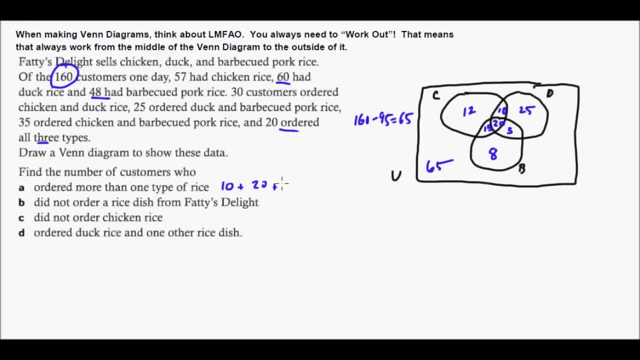 it's going to be 10 plus 20 plus 15 plus 5, which would be 50.. We're good there. Did not order a rice dish. Well, we already did that. That's 65.. Did not order chicken rice, Okay, so did not order. 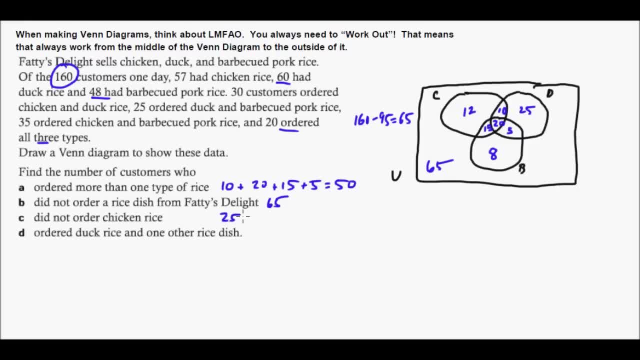 chicken rice. So here's chicken rice, So it's going to be, you know, 25.. You just take everything that's not in there, Plus 5,, plus 8,, plus 65.. Excuse me, So that's. you know the numbers that. 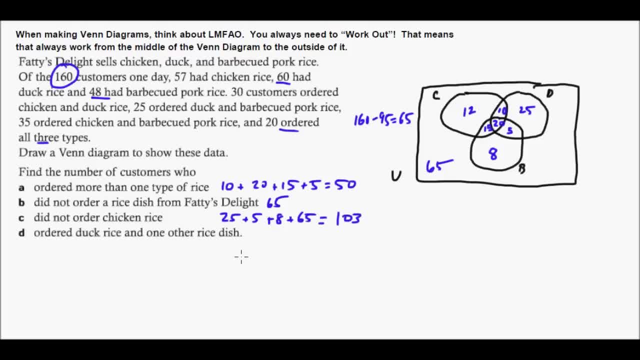 that's going to be 103.. Make sure you count the outside. one In order: duck rice, and one other rice dish. Well, duck rice and one other would be right here and right here. So that's just going to be 10 plus 5, which equals 15.. And you're good to go. So that was pretty straightforward, And let's 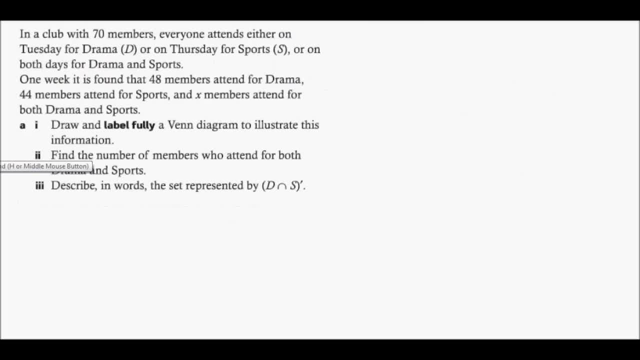 do one last one with a little bit of algebra in it. Okay, it says: in a club with 70 members, everyone either attends. everyone attends either on Tuesday- drama- or Thursday for sports, or on both days for drama and sports. One week it found 48 members. 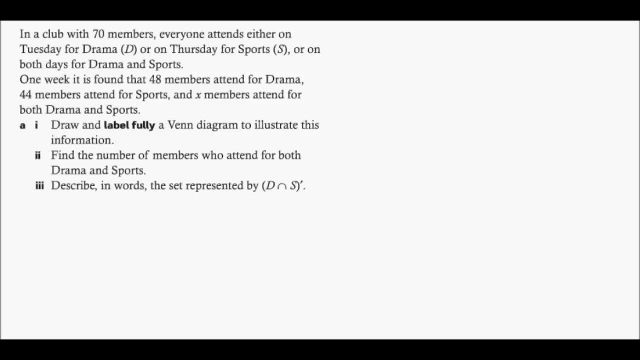 attend drama: 44 attend sports: X. members attend both. Okay, draw and fully label a diagram to illustrate this data. Okay, well, no problem, We have. this is actually only a two circle Venn diagram. We have drama here and we have sports here. So drama and sports. Now they say that the 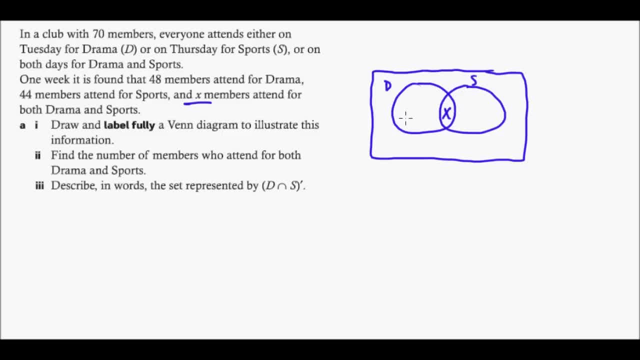 X is. they attended both. So X is going to be, it's going to be here. Now this is where kids get a little confused. Okay, it says 48 attended drama. Well, this is not going to be 48. It's going to be 48 minus X. And then you know sports is going to. 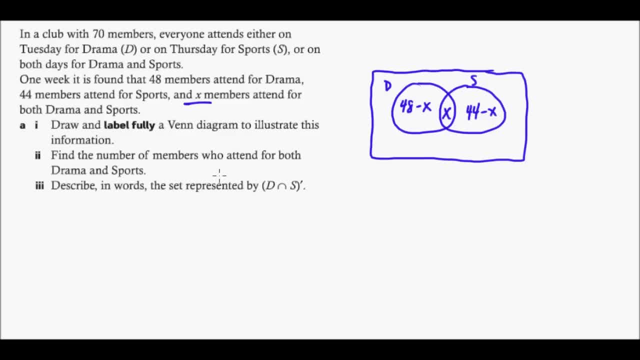 be 44 minus X. Now find the number of members who attended, who attend both drama and sports. Okay, well, you know there's 70 total members here, So we can just use a little bit of algebra: 48 minus X. 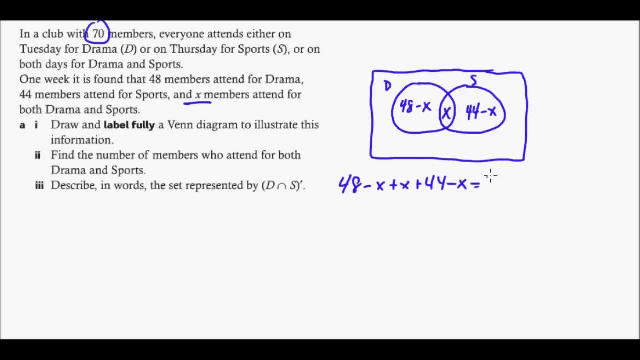 plus X plus 44 minus X 70, so what's this we have? okay, so I'll put these together. so those cancel out. okay, so we get negative X plus 92 equals 70. so we subtract it, we get negative X equals negative 22. well, okay, so X is going to be 22. okay, so the middle is: 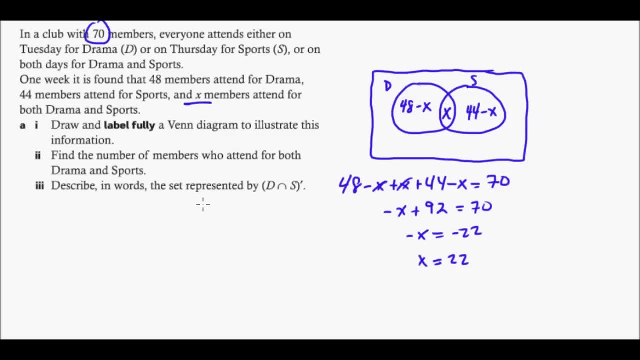 going to be 22, and describing the word in words the sets represent by not D intersection s. so what they're talking about there with not D intersection s is they're talking about this right here and this right here. so this is people who play, did drama only or sports only, okay, and there you go. so event diagrams. 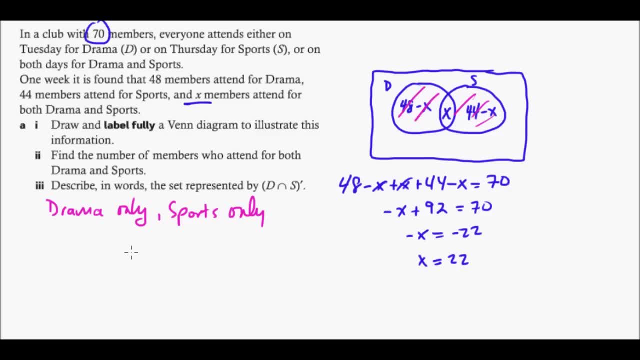 I'm going to do another one with the probability in just a couple minutes, but a you know, if you can get those down, it's some pretty easy marks for you. and you know, don't let the algebra confuse you. sometimes they throw those in there. they can be a little more difficult, but you know it, just remember, like you know, this. 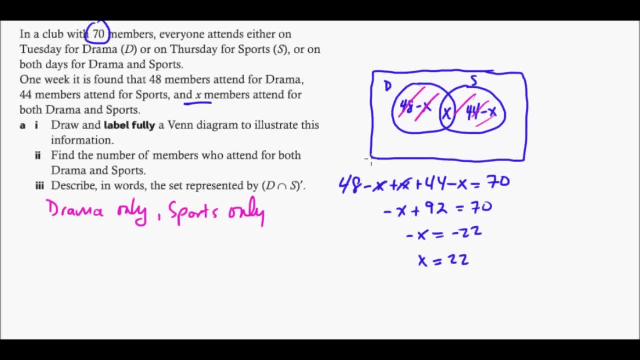 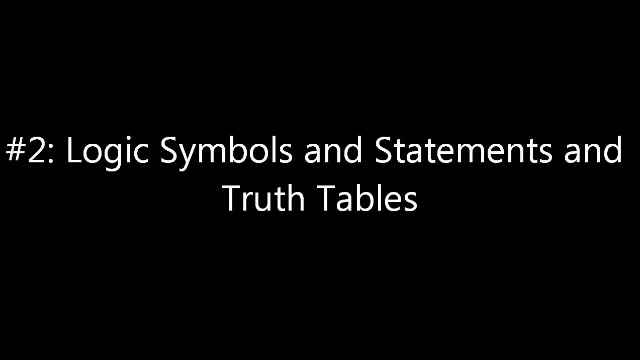 whole thing has to add up to 48. if this is X, you just got to take away X here. that's basically how they always work. anyway, I hope this helped out. we'll move on to the second topic now, logic. all right, so it's going to be aстIt is the second part. okay, so the second section here we. 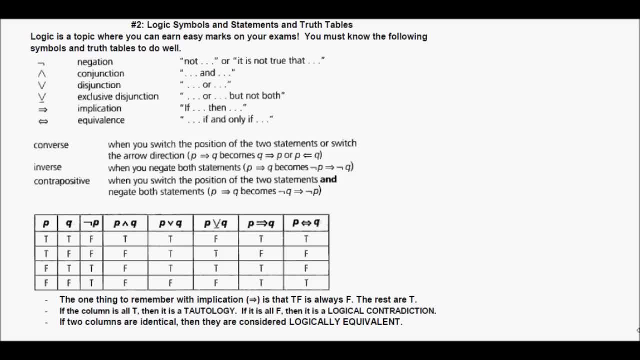 got logic symbols and statements and truth tables the topic where you can earn easy marks. you must know the phone symbols of you know. so this is negation, not this is an. this is just like you know, the logic symbol or not the logic, the set symbol, that looks like that. this is disjunction. this is or-then-or-but-not-both-if-then, if an only if-a-converse is that the mouse is UE10 24. if the mouse is Say I'd rather pick one, it will be a BA관 if you draw ol twenty cent. 웃stopping the question. 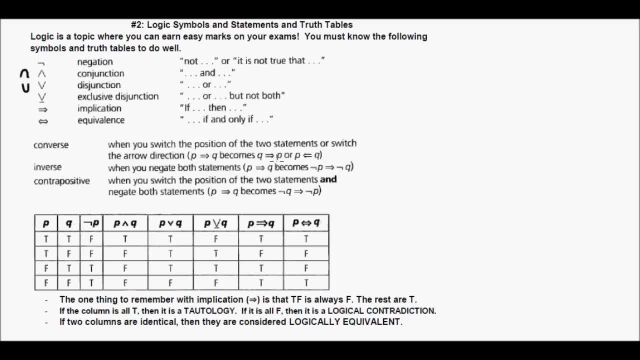 you know, if you have implication of converses, when you just switch them so like P, then Q becomes Q, then P- Inverse means that you negate them both. Contrapositive means that you switch the statements and then you negate them both. You have to memorize this, You just have to. 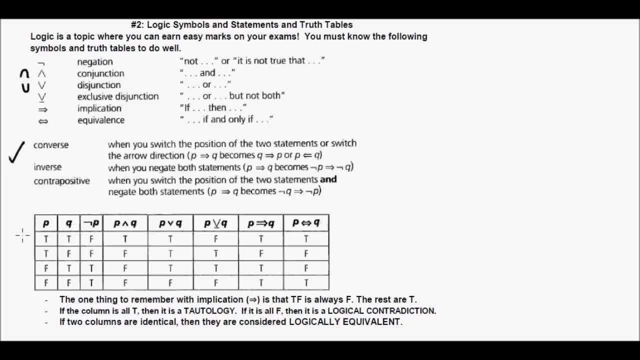 because you're giving away points if you don't. Now here are the most common truth tables. So you know, the thing with and P and Q, it has to be true. true to be true, P or Q, it only has to have one true. So you know, this is the only false right here and this is the only. 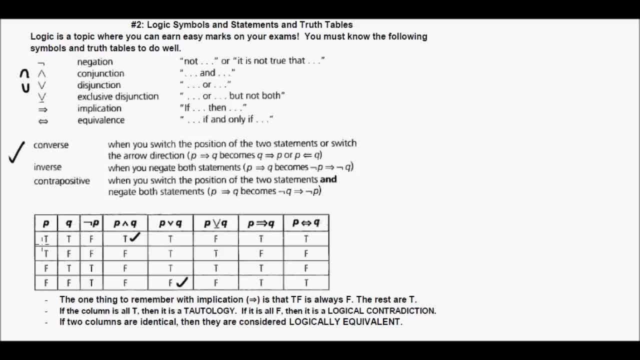 true right here: P or Q, but not both. Well that you know that can only be one, So you're only going to have true on those two. If, then Now the thing with if, then is true, false, True, false. 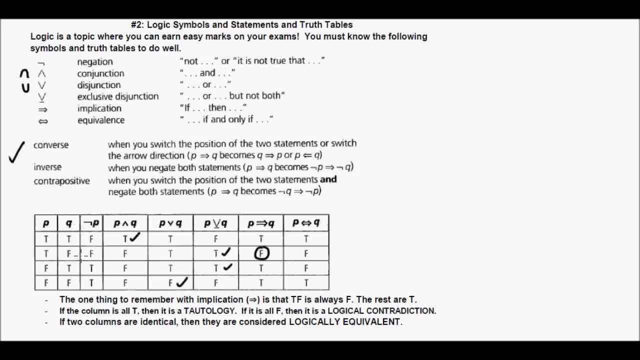 you know, true, false right here. That's never going to work with implication, And then or but not both, That's just going to be true, true or false, false. Okay Now, the one thing to remember with implication is that true, false is always false. The rest are. 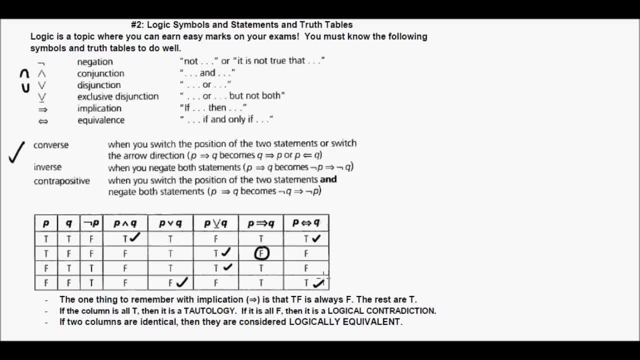 true, And if the column is all true, it's called a tautology. If it's all false, it's called a logical contradiction, And if the two columns are identical, then they are considered logically equivalent. Now, oftentimes, on paper two, they'll ask you one of these: Paper one, paper two. I 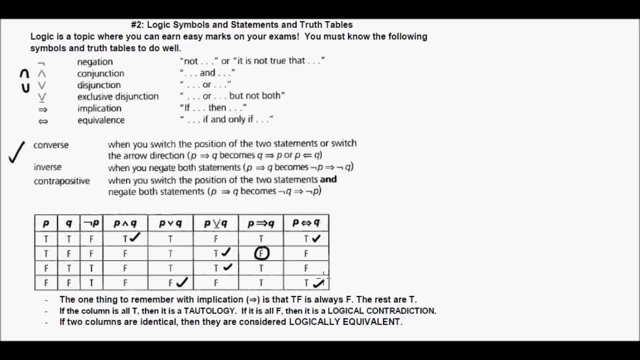 don't know. I've seen them on both And you know they'll ask you to fill in a truth table, And you know, then they'll ask- you know oftentimes it's a tautology- and they'll ask. 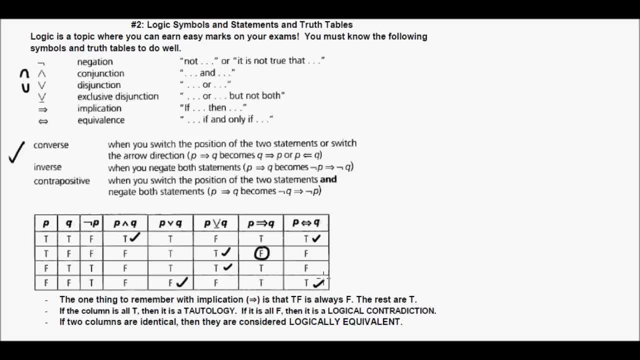 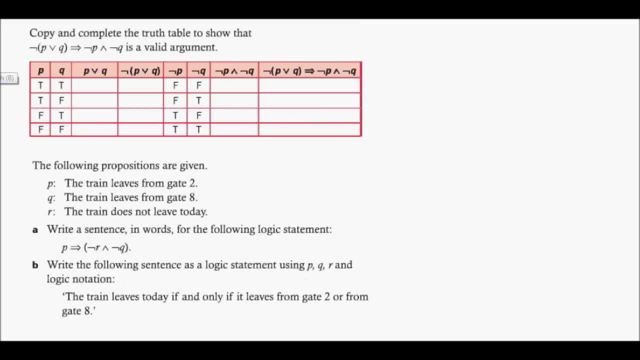 you to do that. So you know, it's really important that you guys know this because it is easy, easy marks, Okay, So let's go ahead and do a problem here. It says: copy and complete the truth table to show that not P or Q. then not P and not Q is a valid argument. Okay, No problem. 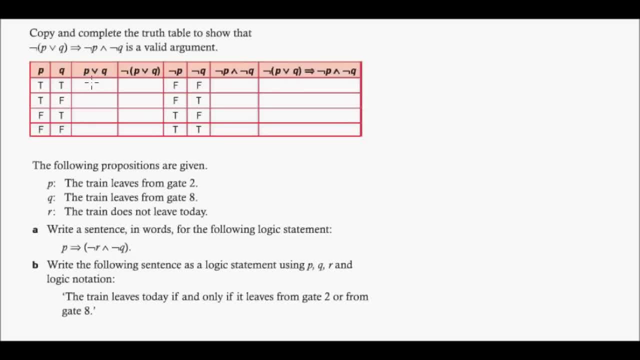 So P or Q. So remember, it only has to be one. So it's going to be, you know, true, true and then false. Now, not that, okay, fine, That's just going to be the opposite of this. So it's. 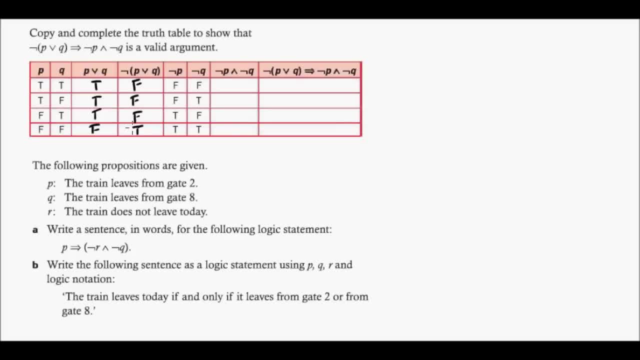 going to be false, false, false, true. Now they do the nots here And remember and has to be true, true. So this is going to be false, false, false and true, And then we go from not okay. 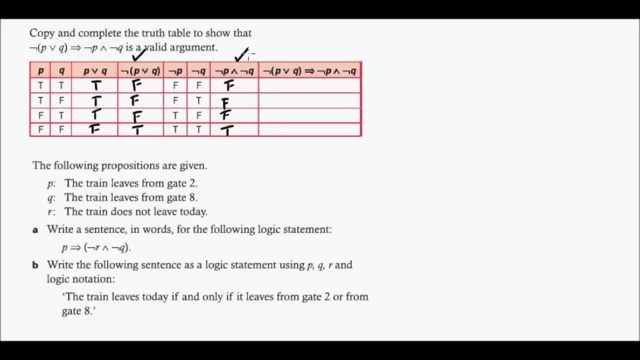 so this column right here, to this column right here, And it's implication. So you know: false, false is true, False, false is true, False, false is true, And true, true is true. Okay, So this is a tautology. 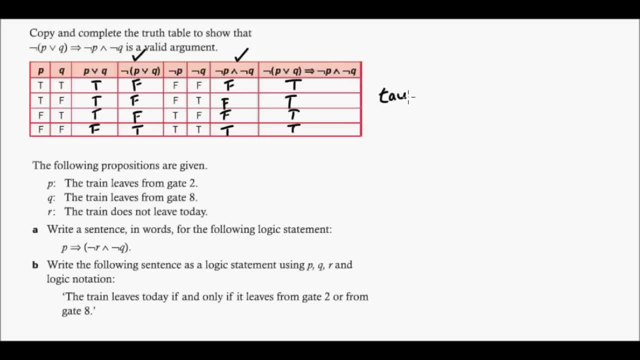 or a valid argument. Okay, So tautology, because it's all true here. Woo, Okay, That was a horrible rocket. Okay, Let's try another one here. It says the following propositions are given: The train leaves from gate two, P, Q. The train leaves from gate eight. The train does not leave from gate. 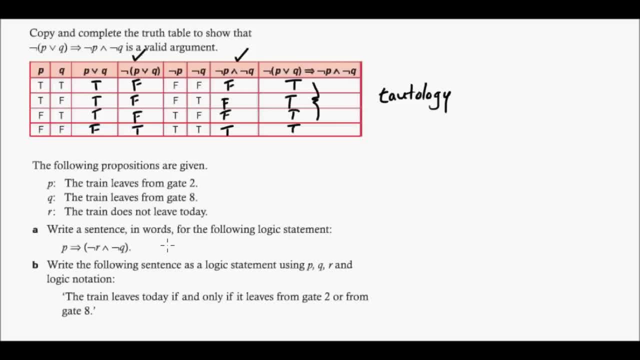 nine And the train leaves from gate nine. The train leaves from gate eight And the train leaves from gate two. Okay, So, remember, anytime you see implication you have to put the if, then So if P the train leaves from gate two, the train leaves from gate two. Okay, Then so if then is. 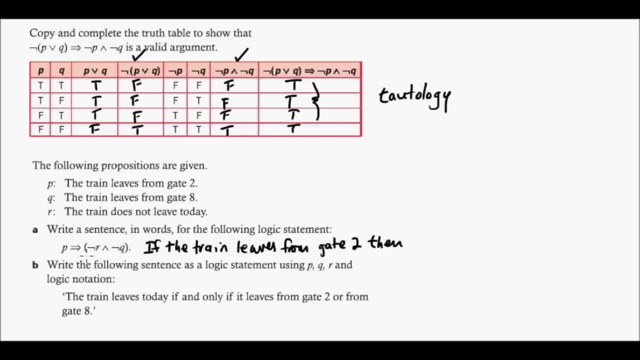 worth one point. That first part would be worth one point as well. Okay, So what does this say? not leaving today? and it's not leaving from gate eight? Um, okay, So then it. um, so if it the train leaves from gate two, then it is does not leave today. So then then it. 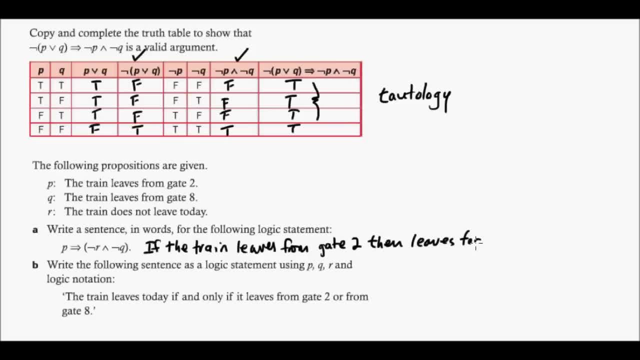 leaves today. So it's not not. that's kind of confusing. And um does not leave from gate eight, I think, Yeah, From gate eight, Okay. So there you go. There's a lot of leeway on those, by the way. So just you know, do the best you can to say what it is, That's. 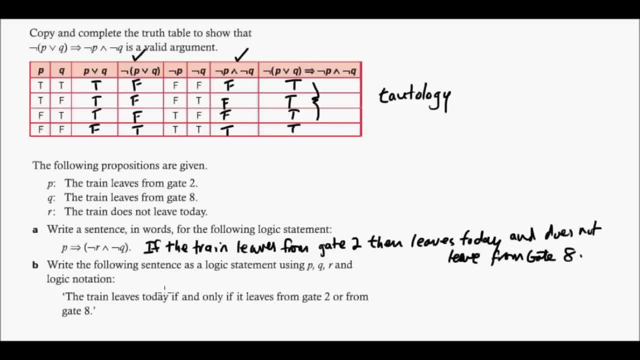 kind of- I don't know, Those are weird. Write the following sentence in a logic argument using PQ and R and logic notation: So if the train leaves today, the train- sorry, the train- leaves today, if and only if. okay, well, if and only if is going to be that it leaves from gate two. So if the 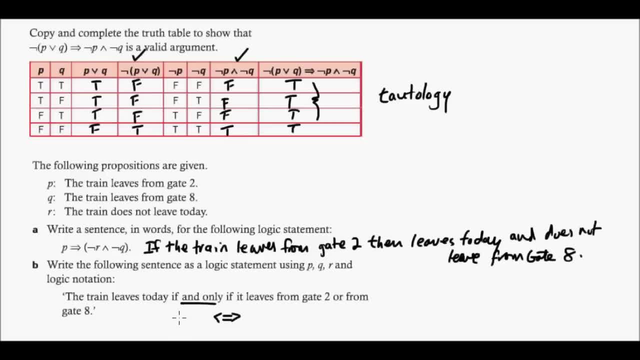 train leaves today: um, so that's going to be not R, and then um, it leaves from gate two or from gate eight, So that's going to be um, P or Q, and make sure that that's here. So let me make sure you put the brackets there in the end, the end of that, and you're. 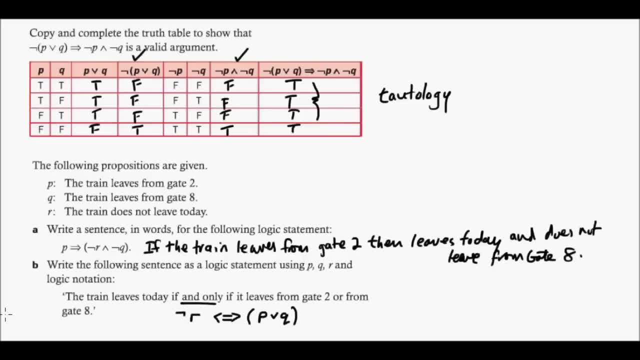 good to go on that. So you know, this is, this is what logic is. Um, you know, and if, if you get good at it and I'll do one more, um, or actually, how many more do I have? uh? 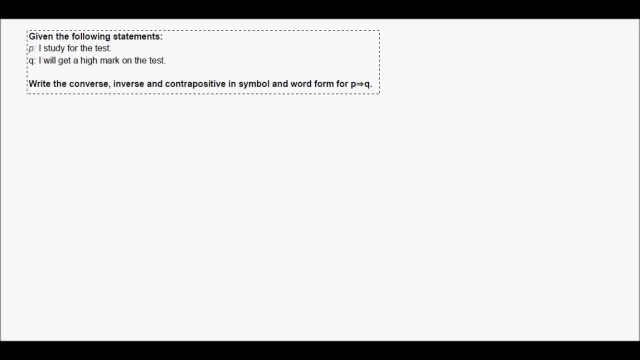 uh, one more, so hold on just a second. Okay, So in the last one here I just want to do some converse, inverse and contra, positive in symbol and word form, just to get going here. So right, The converse, inverse and contra. 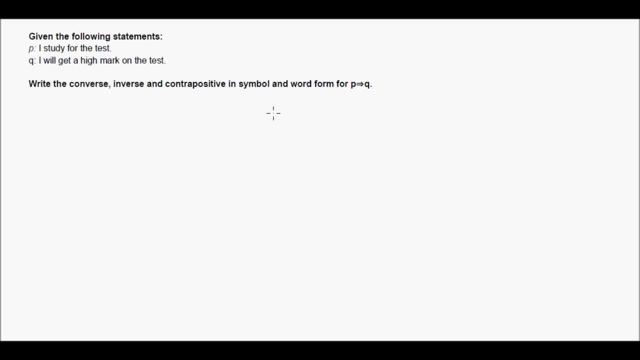 POSM word form for if P then Q. okay, no problem. so the converse is just when you switch it, so it's going to be Q then P. and how would we say that, well, I will get a high mark on the test, or if I will get a high mark on the test, then I, you know? basically, I studied for 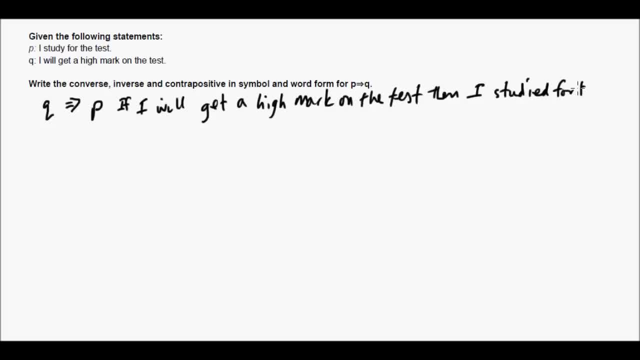 the test. I'm changing the verbiage, I made this one up, so it's not the best one in the world. yep, okay, so the inverse is you, you know you keep the order, but you negate them. so not P, then not Q. so in that case it would be, you know, if I 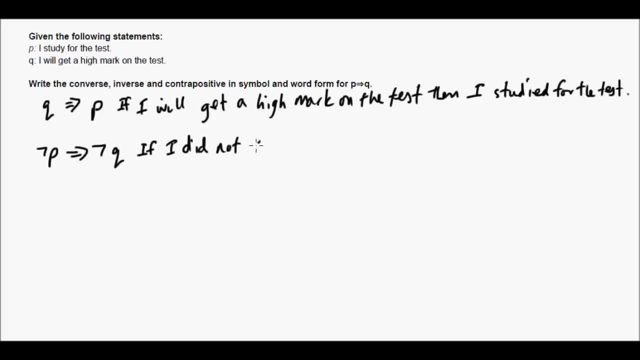 did not study for the test. don't you love my handwriting, it's awesome, huh. then I did not, did not get a high mark, okay, and then finally, you know, we'll switch them and negate them. so not Q, then not P. so that would be if, if. 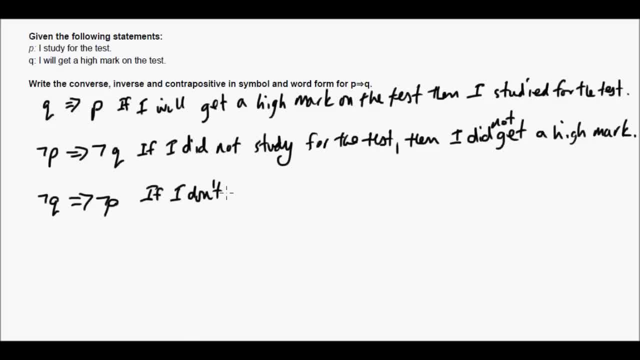 if, if, if I don't get a high mark on the test, then I did not study now. let that be a. then I didn't study now. let that be a lesson for you: study hard, study hard, okay, and you'll get a high mark. okay, anyway, there you go. so you know one might get like a very high mark. you're gonna at the. 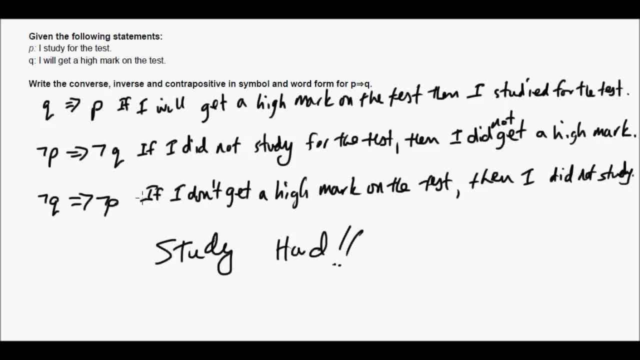 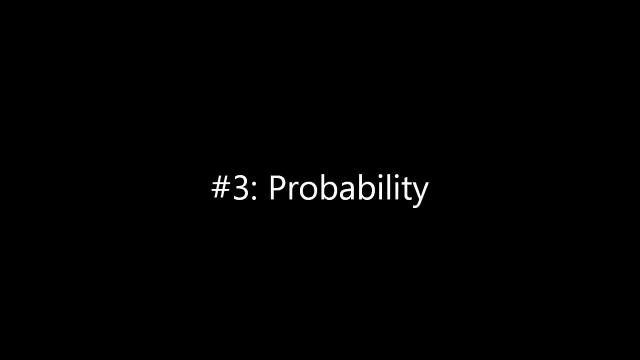 So logic, I have to say it's mostly about memorizing, and it's easy- marks. So you memorize this stuff, you are good to go. All right, let's move on to the last thing: probability. Okay, in this section I'm going to go over probability. 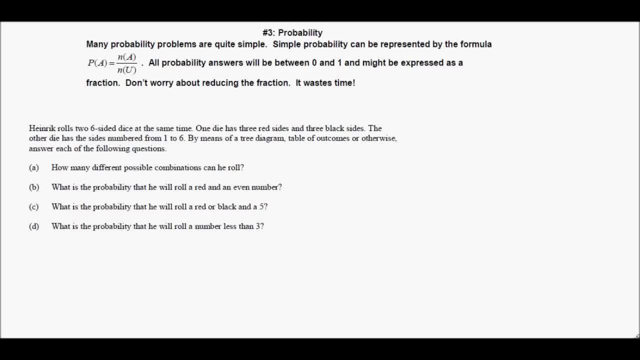 Now I'm going to do quite a few problems on this. Probability comes in a lot of different forms. So you know, if you have some issues with this, I'm going to try and do as many different problems as I can. 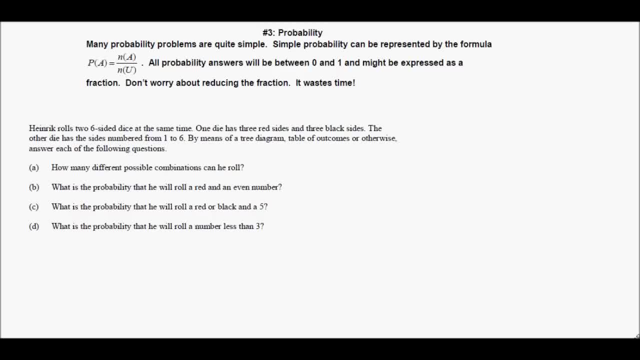 This might take a while, but hopefully it's worth it. Many probabilities are actually quite simple. Simple probability can be represented by the formula: the probability of A equals the number of A over the total number. All probability answers will be between 0 and 1 and might be expressed as a fraction. 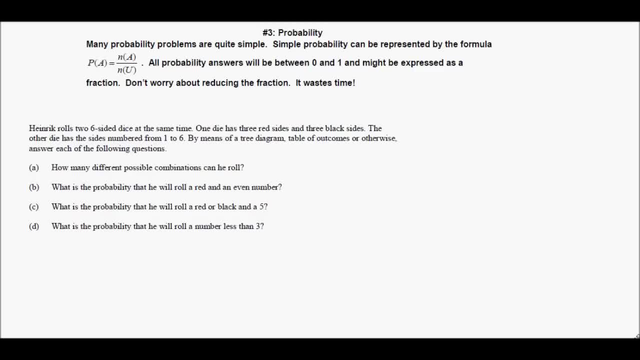 Don't worry about reducing the fraction. So that's one thing where kids kind of make some mistakes: They get the right initial fraction, then they reduce it wrong and it's just a waste of time. So let's look at an example, a pretty straightforward one here. 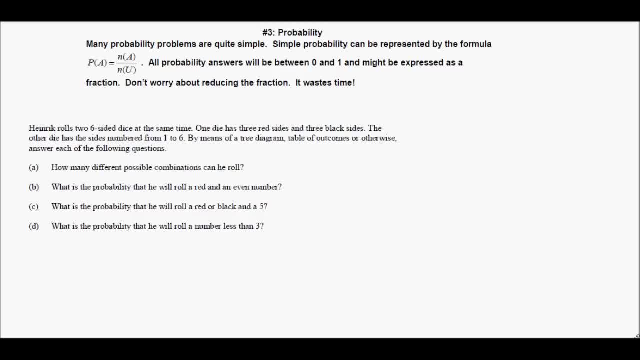 It says Heinrich rolls two six-sided dice at the same time. One die has three red sides and three black sides, The other is from 1 to 6.. By means of a tree diagram, take all of outcomes or otherwise. answer the following questions. 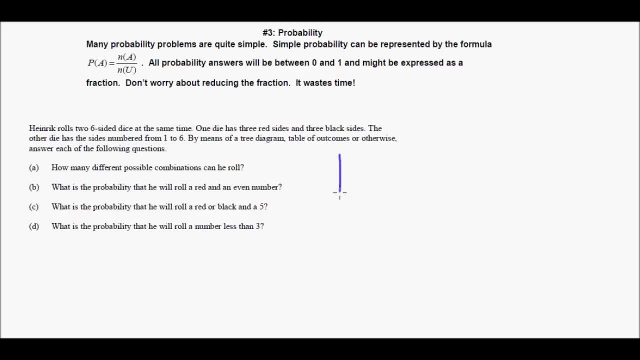 Okay, well, this one, you're best off making a grid. I think, personally, That's an awesome line right there. That is horrible, Okay. So you know, die one here. you know you have red and you have what. is it black? 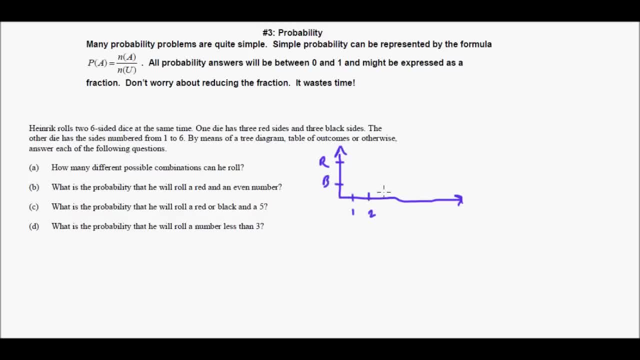 Okay, black. And then you have 1 through 6 here, Okay. Now, a common mistake kids made on this is they put three reds and three blacks, and that's actually not red or black doesn't matter, It's the same outcome. 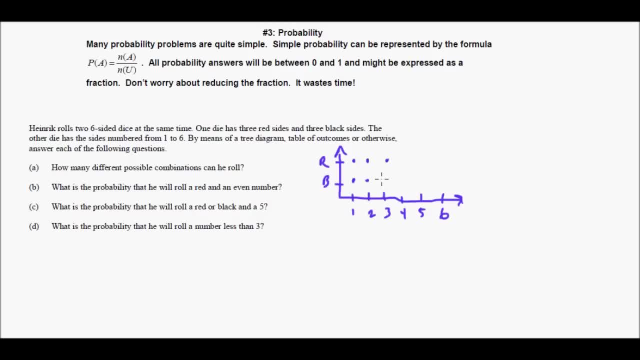 So it doesn't matter which red or black you get. Okay, there's only two outcomes. So if you draw the little dots here, And how many outcomes, How many outcomes are there? Well, there's 12.. A lot of kids in this problem. I gave this to my kids in a test and they put 36.. 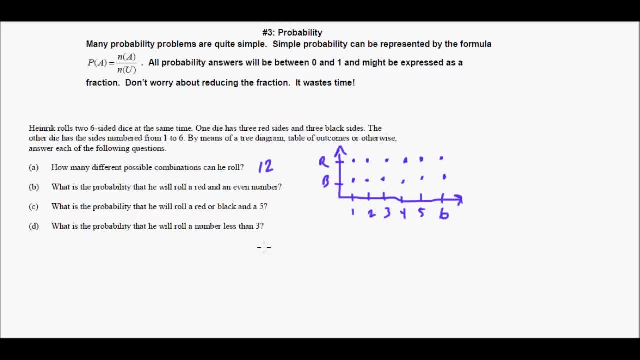 The answer is 12.. What's the probability? you roll a red in an even number. Okay, well, let's use a red pen for that. A red in an even number? Well okay, here's red. and then here's even numbers 2,, 4, and 6.. 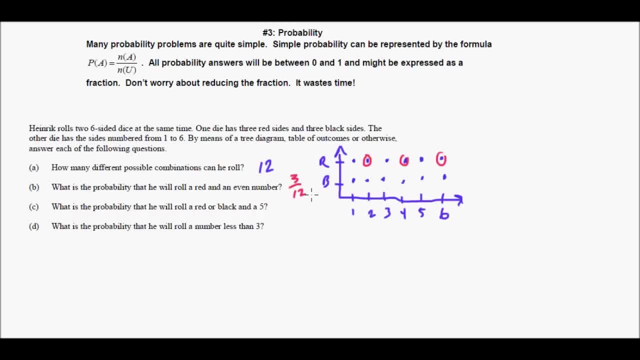 So that's just going to be 3 out of 12.. Okay, What about red or black and a 5?? Okay Well, red or black and a 5, well, it has to be a 5 here and it's red or black. so that's just 2 out of 12.. 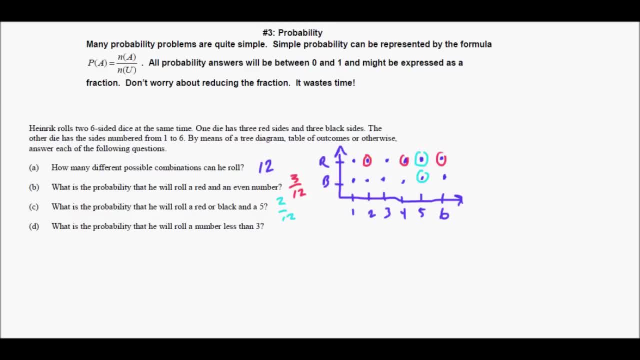 And again, don't reduce them. What's the probability it rolls? a number less than 3? Okay, well, a number less than 3 is just 1 or 2, so it's going to be that one, that one, that one and that one. 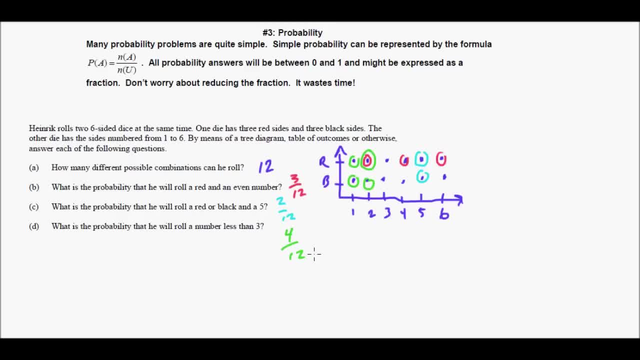 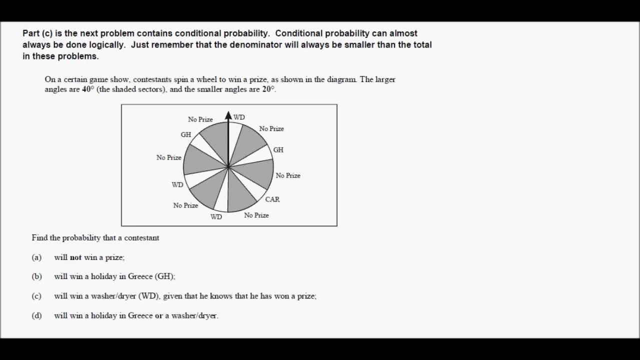 Well, that's 4 out of 12.. Boom done, Easy, Okay, so that's simple probability right there, Let's do another one. Okay, so it says part C in the next problem contains conditional probability. Conditional probability can almost always be done logically. 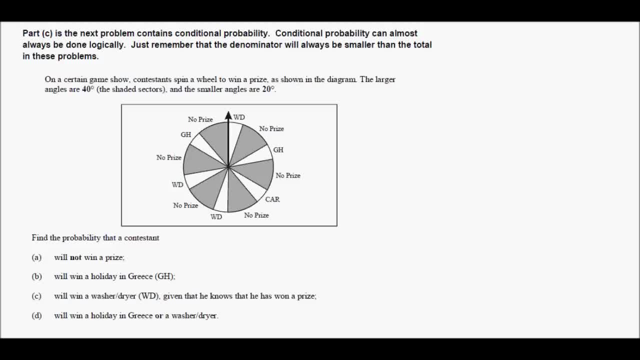 Just remember that the denominator will always be smaller than the total in these problems. Okay, no problem, We'll get to that in a second. It says: on a certain game show, contestants spin a wheel to win a prize. It's shown in the diagram. 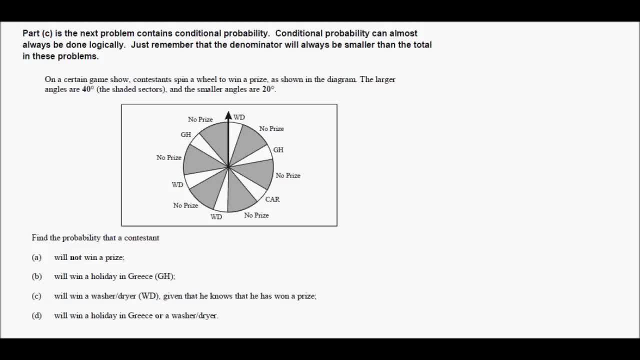 The larger angles are 40, the shaded sectors and the smaller angles are 20.. Okay, no problem. Now the thing you've got to know here is that a circle has 360 degrees in it, right, Okay? so find the probability that a contestant will not win a prize. 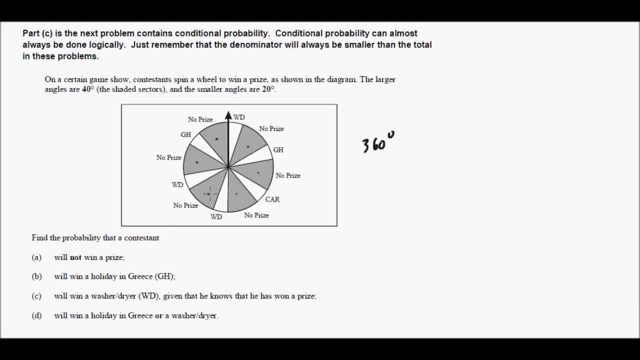 Well, that's going to be 1,, 2,, 3,, 4,, 5, 6 times 40,, which is 6 times 40 is 240.. So it's going to be 240 out of 360, and you just leave it. 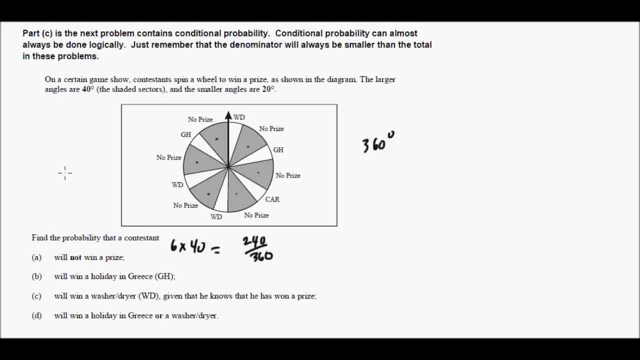 Don't even reduce it. We'll win a Greek holiday. Okay, we'll win a Greek holiday. Let's see, Greek holiday is right here and right here. Are there any more? No, and those are 20.. So 2 times 20 is 40.. 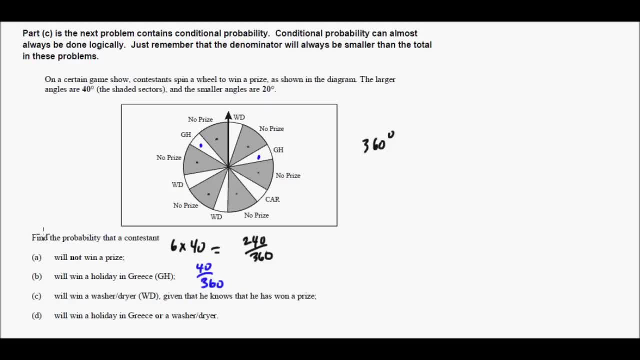 So that's going to be 40 out of 360.. Okay, now here's conditional probability on the next one. okay, So it says we'll win a washer-dryer, given that you know he's won a prize. Okay, well, how many prizes do we have here? 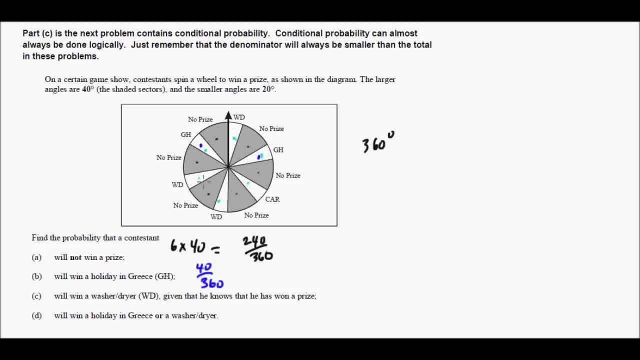 We have 1,, 2,, 3,, 4,, 5, 6.. So our denominator is 6 times 20,, which is 120.. So that's going to be on the bottom. Now, which one of those are washer-dryers? 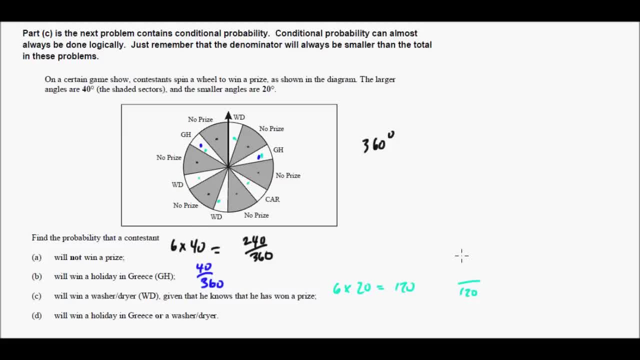 How many are there? There's 1,, 2, 3.. So it's going to be 3 times 20.. Which would be 60 out of 120, and you're good to go on that. and then the last one. 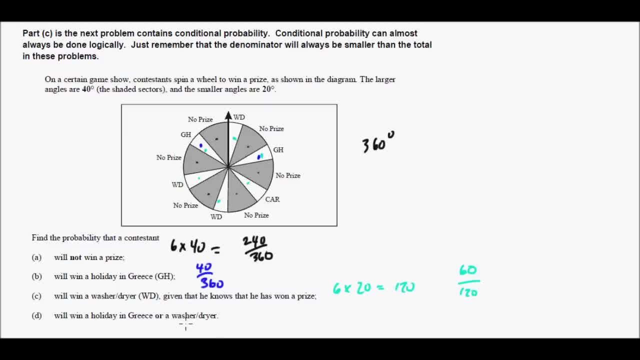 again is you just have to add two things. Now, this isn't conditional probability. It goes back to mean simple probability: We'll win a holiday in Greece or a washer-dryer. Well, okay, so holiday in Greece or a washer-dryer. 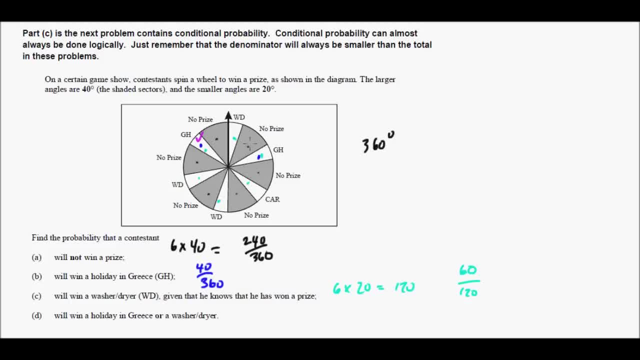 Let me get a different color for that. So Greek holiday washer-dryer, Greek holiday washer-dryer, washer-dryer, You know. So they don't get the car. Oh too bad. So 5 times 20 is 100 over 360.. 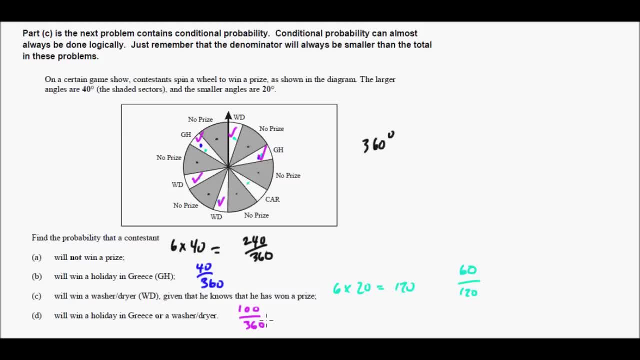 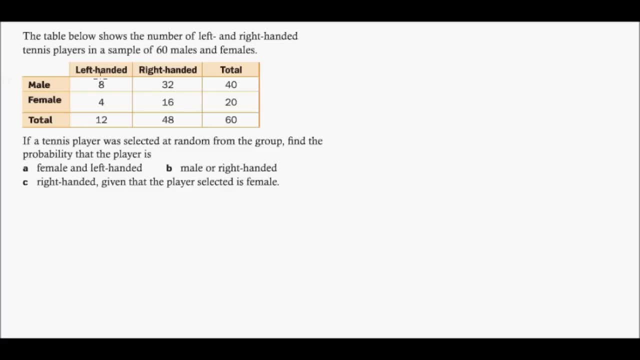 Okay, so that takes care of simple probability. Let's move on now to some independent probability. Okay, I want to do one more simple probability, and this one's from a table. The table below shows the number of left- and right-handed tennis players. 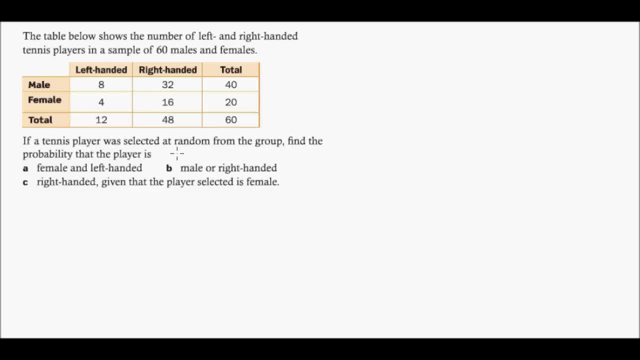 in the sample of 60 males and females. If the tennis players are selected random from the group, find the probability of the female and left-handed Okay. well, left-handed female is right here, So that's just going to be, you know, 40 out of 60, or it's not 40,, 4 out of 60,, excuse me. 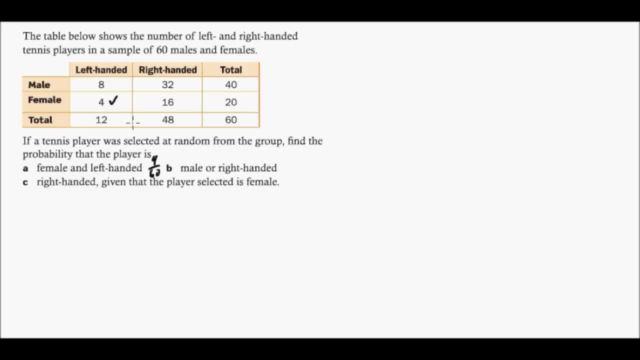 All right, and let's look at B: male or right-handed. Now, male or right-handed, you have to be careful with this. So male is going to be this and this, but you also have to count the female right-handed. 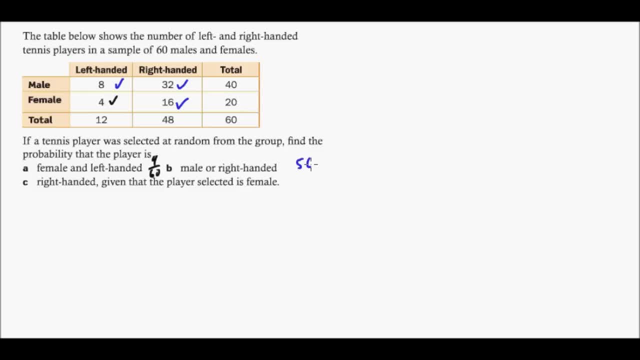 So 32,, that's 48, and that's going to be 56 out of 60.. Okay, And then right-handed, given that the player is female. Okay, so this again is conditional probability. So let's look at female here and right-handed, so that's just going to be 16 out of 20.. 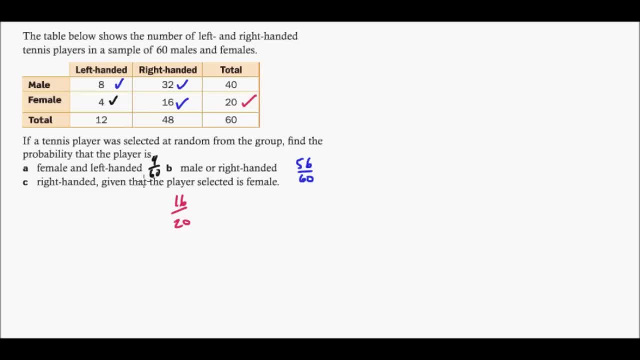 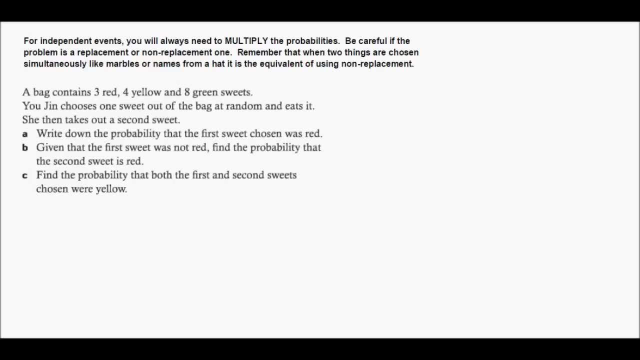 So you know it's in conditional probability. you know the denominator is always getting smaller there. That's all you have to remember about it. Okay, now we're going to go on to independent probability. Okay, for independent events, you will always need to multiply the probabilities. 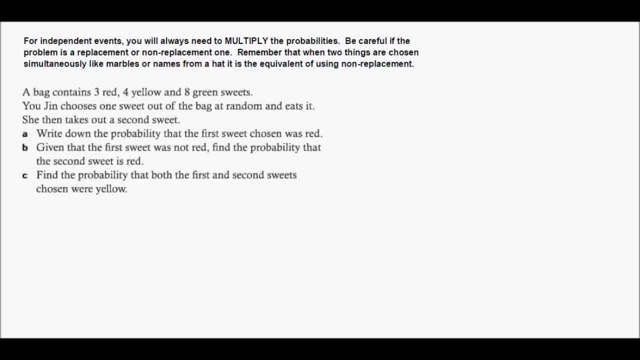 Be careful: if the problem is a replacement or non-replacement one, Remember that when two things are chosen simultaneously, like marbles or names from a hat, it is equivalent of using non-replacement. So when you do use non-replacement, that means that the you know. 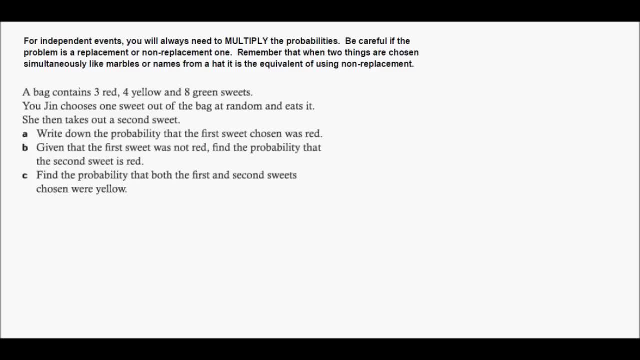 numerator and the denominator are going to get smaller by one. the next time you do it usually. Okay. Well, the denominator for sure by one. Let's do a couple problems. A bag contains three red, four yellow and eight green sweets. 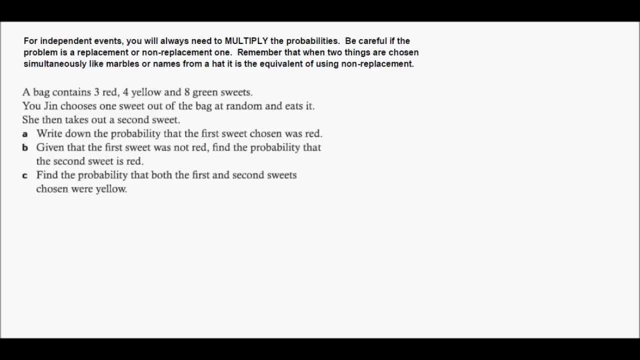 Yujin chooses one sweet out of the bag, random, and eats it. Then she takes out a second sweet. Write down the probability that the first sweet chosen was red. Okay, well, that's easy. There's 15, and that's three out of 15.. 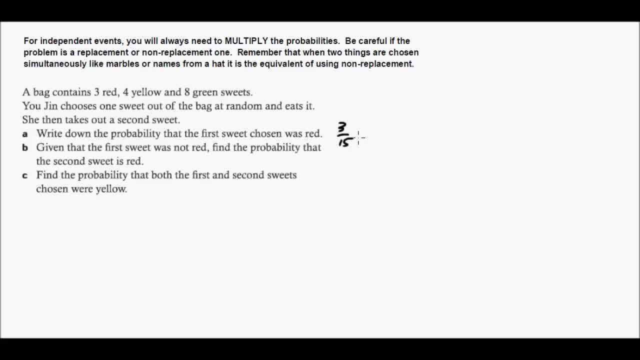 That's no problem, It's not a big deal. Again, that's simple probability. Given that the first sweet was not red, find the probability that the second sweet is red Okay. well, again, this is conditional probability- that she took one out and she ate it. 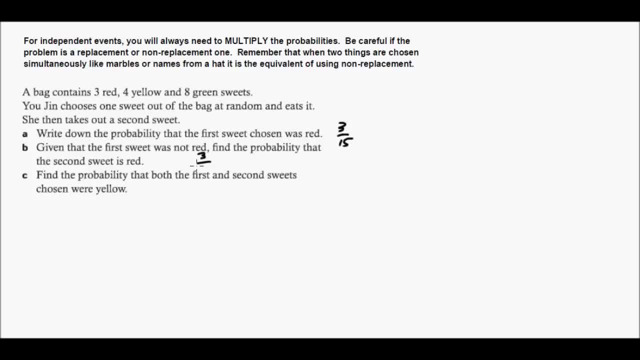 It was either yellow or green, So there's still three red ones left, but at the end there's only 14, because she ate one of them. Now, this is what I'm more concerned with here: Find the probability that the first and second sweets were both yellow. 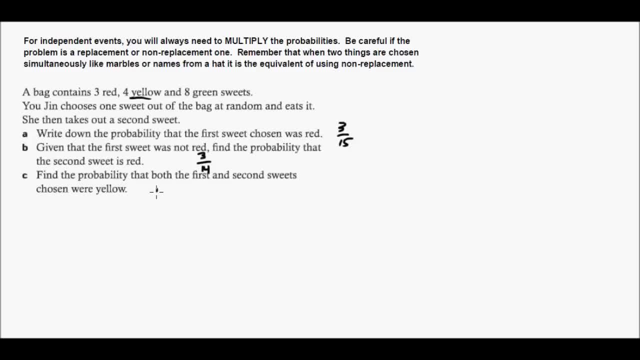 Okay, well, there's four yellow sweets, right? So when she grabs the first one, the chance is four out of 15.. And then you need to times it, or multiply it by times it. What am I in second grade? 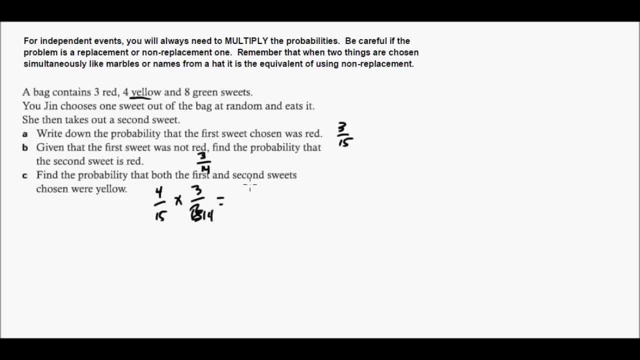 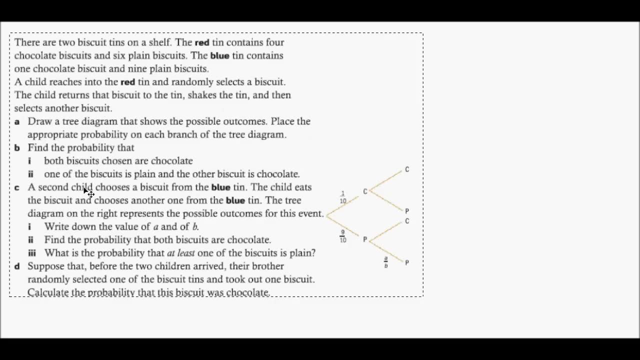 It's not 15.. It's 14.. Okay, so that would be. you know, find the probability that first and second sweet chosen were yellow. Yeah, so it would be 12, and then this would be 210.. Okay so, yeah, just sorry for the delay there. 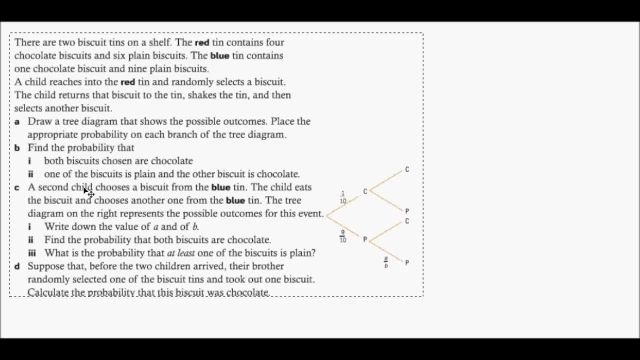 Not that there was much of a delay, but I just realized I made a mistake on my Answer sheet I gave my kids. That's not good. Okay, there are two biscuit tins on a shelf. Okay, this one. we're going to use a tree diagram, which is good. 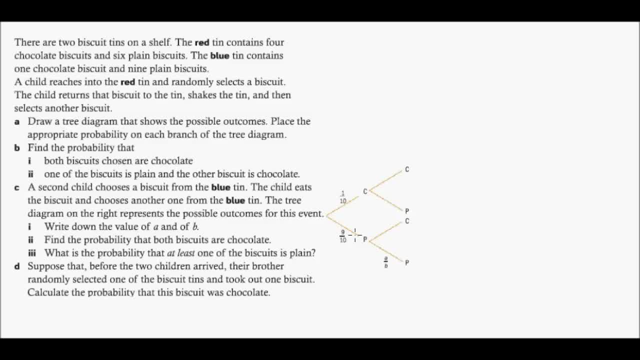 Okay. the red tin contains four chocolate biscuits and six plain biscuits. The blue tin contains one chocolate biscuit, nine plain biscuits. A child reaches into the red tin, randomly, selects a biscuit. The child returns the biscuit to the tin, shakes the tin, then takes another biscuit. 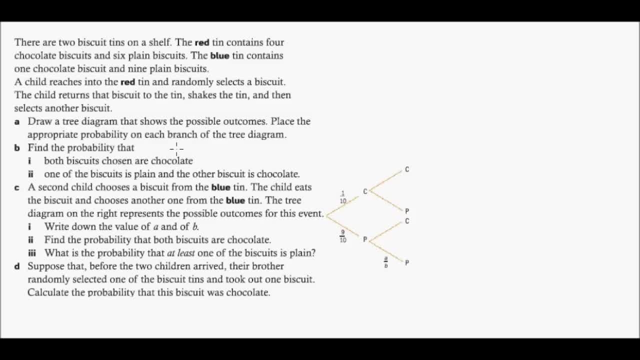 Okay, that's gross, but that's all right. So draw a tree diagram that shows the possible outcomes. Place the appropriate probability on each branch. Okay, so we're talking about the red tin here. So what are our choices? We have, you know, chocolate and we have plain. 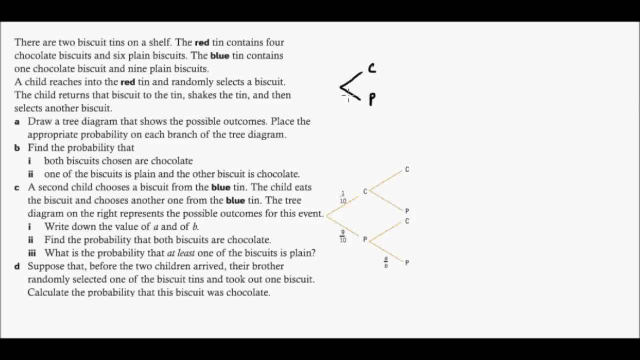 Okay. so how many chocolate are there? There's four chocolate and six plain. So probability of a chocolate is four out of ten. Probability of plain is six out of ten. Now the kid puts it back. for some reason I've never seen a kid put a biscuit back, but you know, whatever. 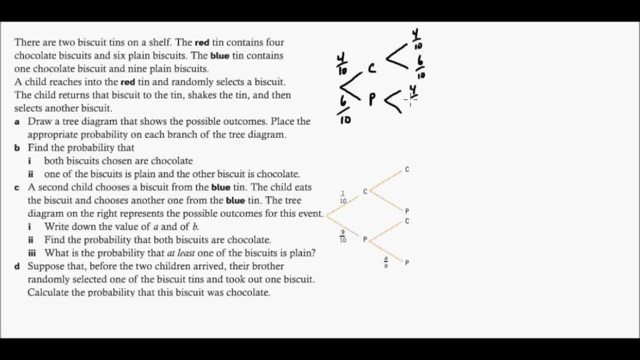 Four out of ten, six out of ten, and then four out of ten, Six out of ten. So this is basically non-replacement probability. Okay, and so we got no problem. we got that done. Find the probability that both are chocolate. 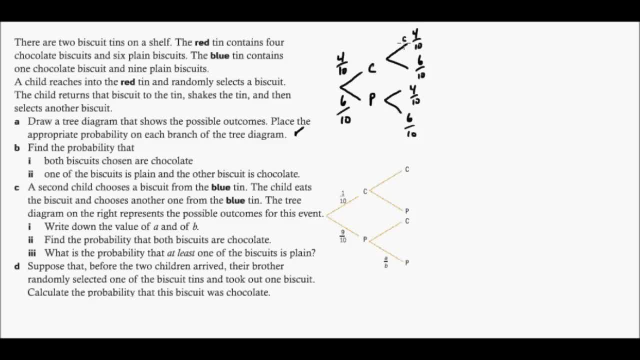 Okay, well, we'll just do. I should have written chocolate plain, chocolate plain. So we just go: chocolate chocolate, which would be, you know, four-tenths times four-tenths, which is 16 over 100.. 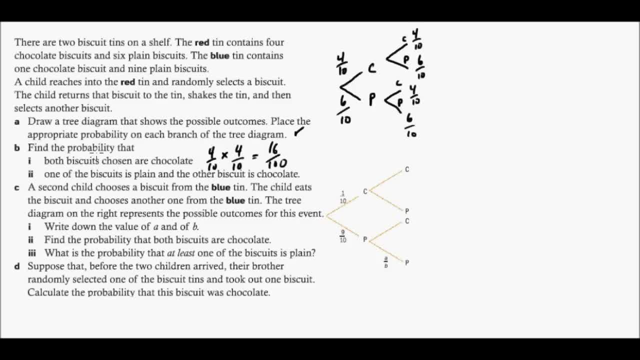 Okay. And then part two: one of the biscuits is plain and the other biscuit is chocolate. Okay, this is where they try and confuse you a little bit. So one biscuit is plain and the other is chocolate. Well, we're going to have to add two probabilities here. 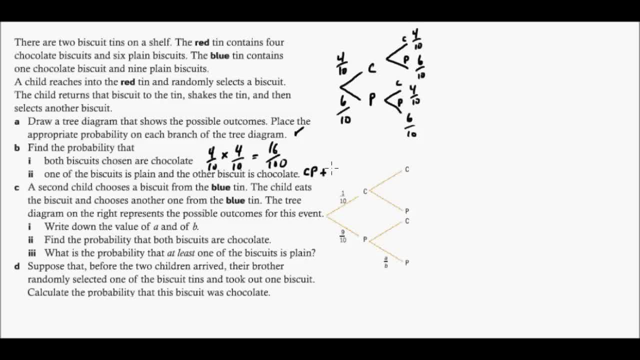 We can have chocolate plain plus plain chocolate. Okay, so you know, we'll just go. I'll move it over here a little bit. Four over ten times six over ten plus four over, or not six over ten Times four over ten. 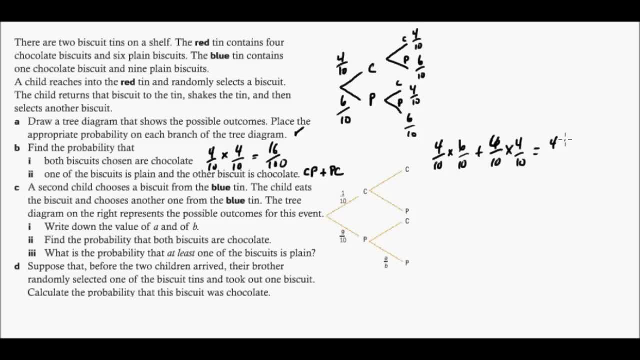 And that's just going to be, you know, 24 over 100 plus 24 over 100, which would just be 48 over 100. So that's where you're adding two probabilities together. Okay, Now a second child chooses a biscuit from the blue tin. 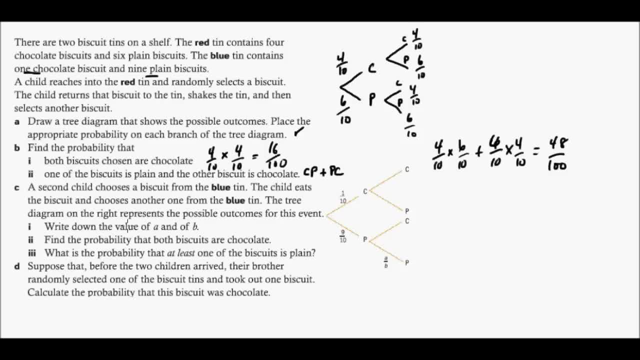 Okay, what do they have? Blue one chocolate, nine plain. Okay, no problem. The child eats the biscuit. Okay, that's more like it. They're more likely to eat it, I think- And chooses another one from the blue tin. 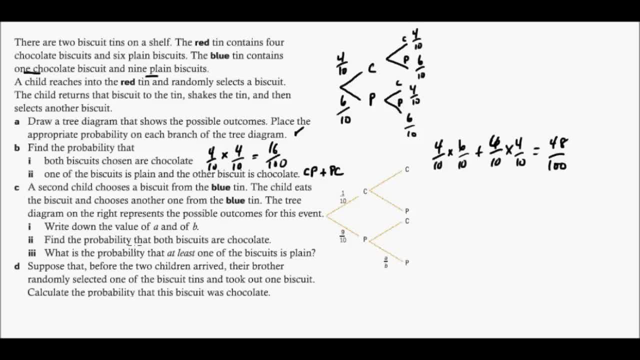 Okay, no problem. The tree diagram represents possible outcomes, the event, So write down the values of A and B. Okay, well, okay, so let's do this. One chocolate, nine plain. Well, if they eat a chocolate, there's going to be zero left. 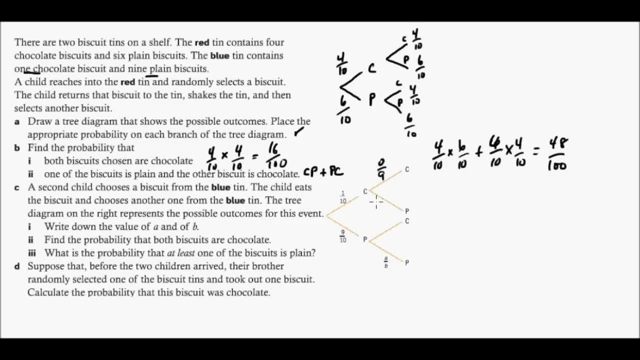 There's going to be zero out of nine, And then this would be nine out of nine. I just like filling in the whole thing. I think it's easier If they eat a plain one. it would be eight out of nine, And then this would be one out of nine. 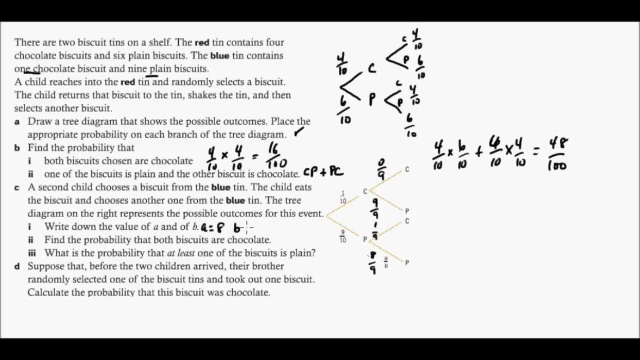 So you know, A equals eight and B equals nine. Okay, Now find the probability that both biscuits are chocolate. Well, there's only one biscuit, so both biscuits can't be chocolate, So that probability is zero. At least one of the biscuits is plain. 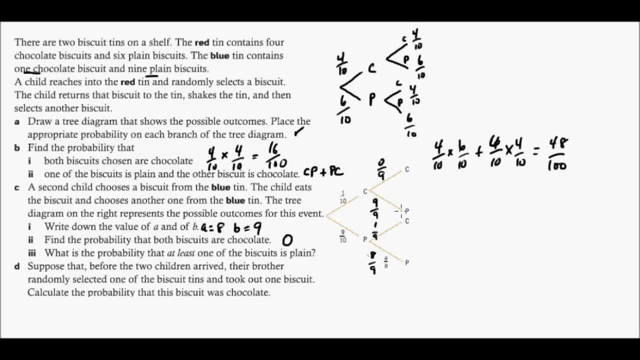 Well, again, you know, look this one, this probability: chocolate, plain, plain chocolate and plain plain, Those are all. But since you can't have chocolate chocolate, it has to have one biscuit that's plain. So the probability there is actually going to be one. 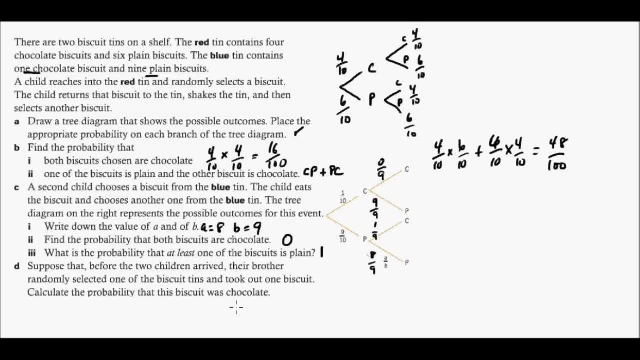 Now suppose that before the two children arrived, their brother randomly selected biscuit tins and took one biscuit. Calculate the probability. the biscuit was chocolate, Okay, now this one. okay, you have to whenever they say randomly selected. okay, so we have the red tin and we have the blue tin. 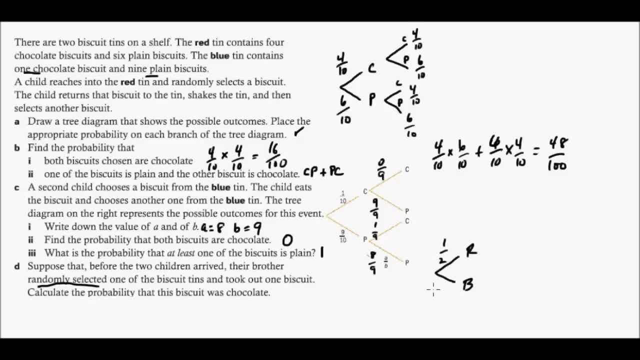 So randomly selected, means that there's a half probability of taking each. Now for the red, we have to do what's chocolate and plain and chocolate and plain. So for the red one, it was what? four out of ten and six out of ten. 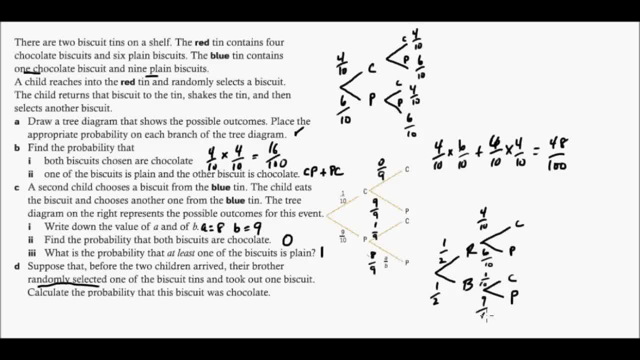 And this was one out of ten and nine out of ten. Okay, so you know, calculate that both biscuits are chocolate. Okay, no problem, We can do that. So we'll just do, you know, one half times four tenths plus one half times one tenth. 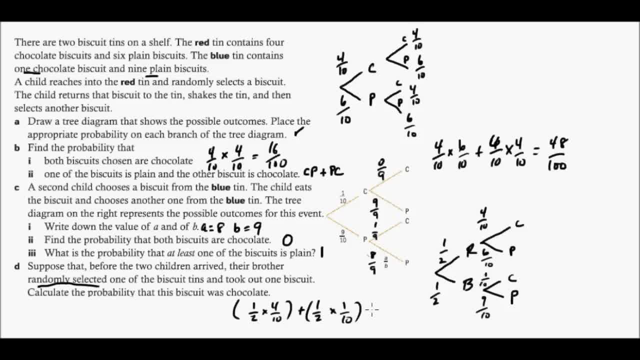 So that's, you know, four twentieths plus one twentieth, so that's going to be five twentieths, And there you go. Okay, so that's a tree diagram problem. That's a pretty good one, because it has independent probability. 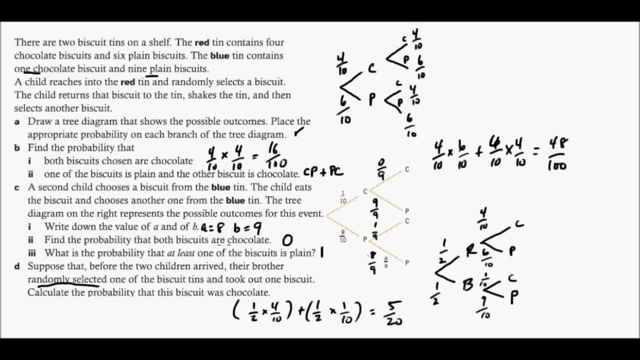 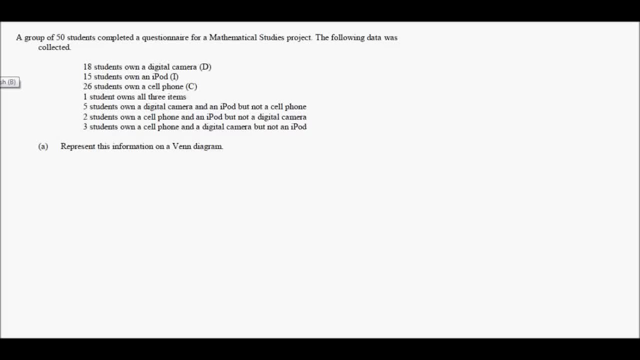 It has replacement, not replacement. Not bad, All right, let's do one last problem, One more, Okay. this last problem says a group of fifty students completed a questionnaire for a mathematical studies project. The following data was collected: Eighteen students own a digital camera, iPod, fifteen iPod. twenty-six own a cell phone. one owns all three. five owns- okay, digital camera but not a cell phone. two owns a cell phone. blah, blah, blah, blah, blah. 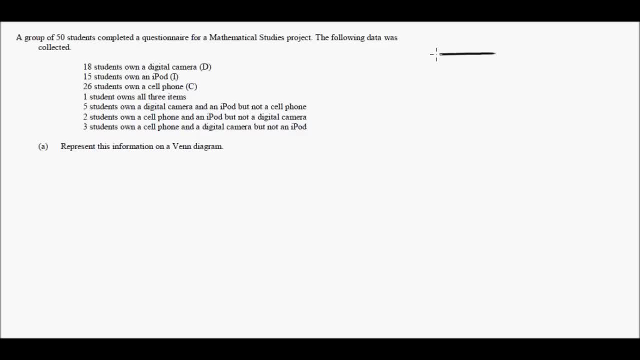 Okay, no problem, Represent the information on the Venn diagram. So let's bust out a Venn diagram here really quickly, Okay? So remember, you have your universal set here and we have three horrible circles, as always. And let's see D- digital camera- I would be- iPod- and C- cell phone. 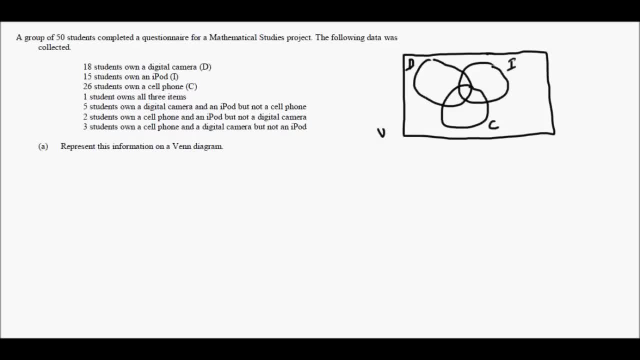 Okay, no problem, Let me switch up some colors here so we can see what's going on. Remember, always work out. So one person owned all three items, so one right there. Five people owned a digital camera and iPod, but not a cell phone. 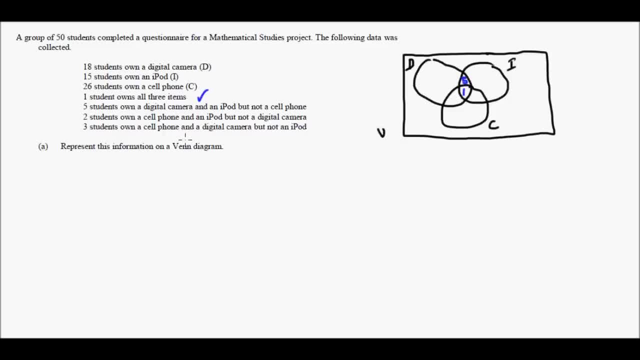 So five is going to be right there. So this is actually a pretty easy Venn diagram. You don't need to subtract. Two owned a cell phone and iPod- okay, so that's, but not a digital camera. And three people owned a cell phone and digital camera- okay, so that's right there. 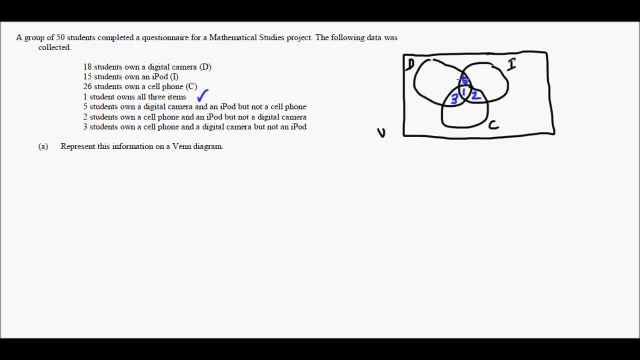 Now, eighteen people owned a digital camera. Well, that's eight. nine, so that's going to be nine. right there, How many people owned iPod? Fifteen, so that's seven. eight, so that's going to be seven. 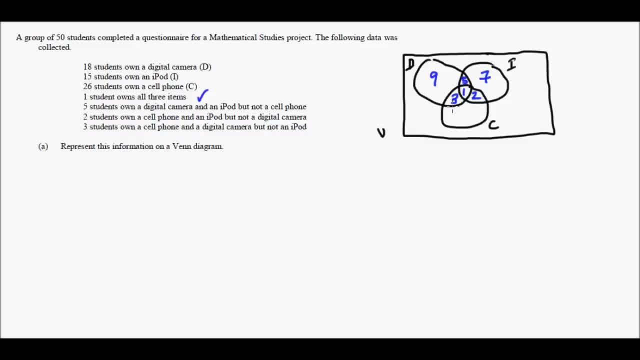 And then twenty-six owned a cell phone. Twenty-six owned a cell phone. Okay, well, that's six, so that's going to be twenty. right there, Okay, and you know, let's see, That's fourteen, twenty-one, twenty-two, twenty-four, twenty-seven and forty-seven. 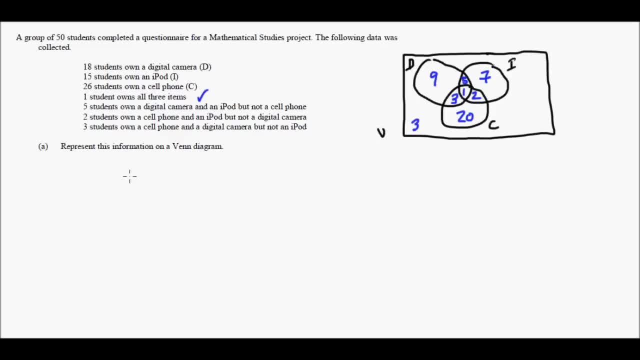 So that means three didn't own anything at all. Okay. so let's look at some of the rest of the problem. Hold on just one second, Okay. so part B here says calculate the number of students who own none of the above items. 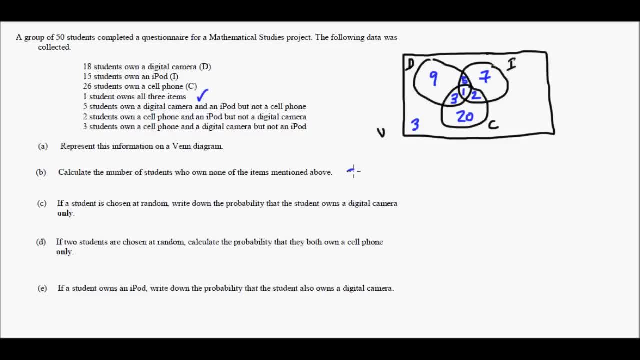 Well, we already did that. We subtract all of them from fifty, so the answer there is going to be three. If the student is chosen at random, write down the probability that the student owns a digital camera only. Well, that's nine right there. so that's just nine out of fifty. 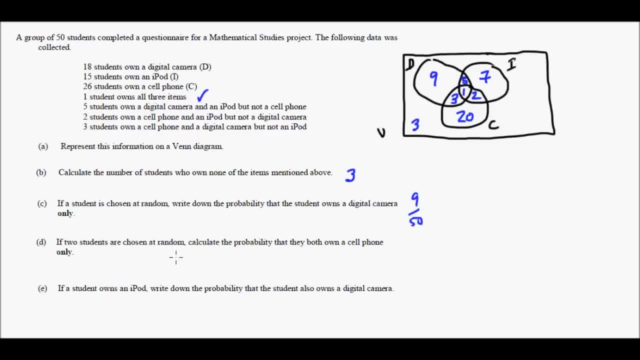 Now, if two students are chosen at random, okay, this is independent probability. Calculate the probability they both own a cell phone only. Okay, well, that would be the first student would be twenty out of fifty. Now, assuming we choose the first student, then the next one would be nineteen out of forty-nine.